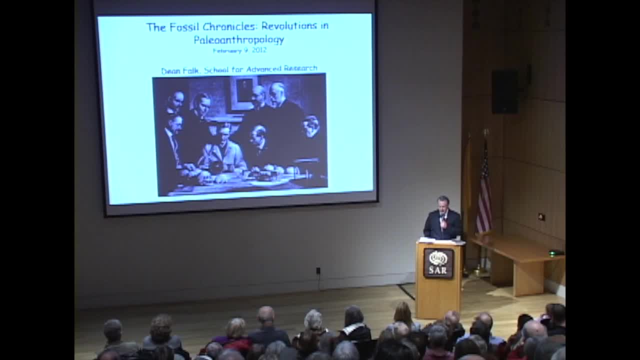 since 1997 and was elected to the American Academy for the Advancement of Science in the year 2000.. Let's welcome Dr Falk and hear about her work. Thank you, James, For that very nice introduction. it's really gratifying to see so many people out and interested. 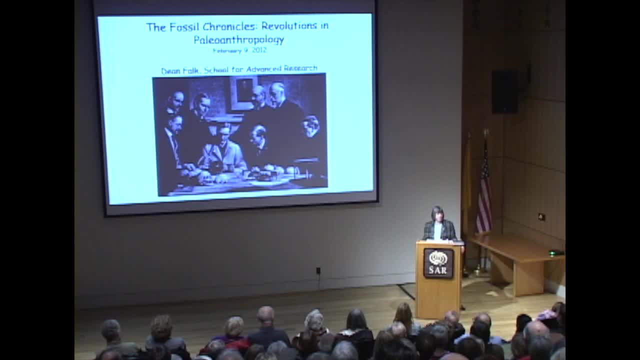 in paleoanthropology. I spoke here some years ago about a discovery called Homo floresiensis, otherwise known as hobbits, And one of our colleagues at SAR- somebody who's very active on the board- told me that during the middle of the talk. 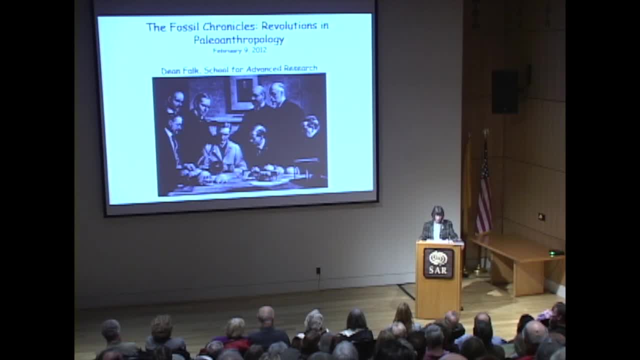 my father got up with his two children and they left. And she heard the children saying to the father: but dad, you said this was about hobbits. So fair warning, I'm so happy to see some young people here And I will be talking about hobbit, but maybe not the. 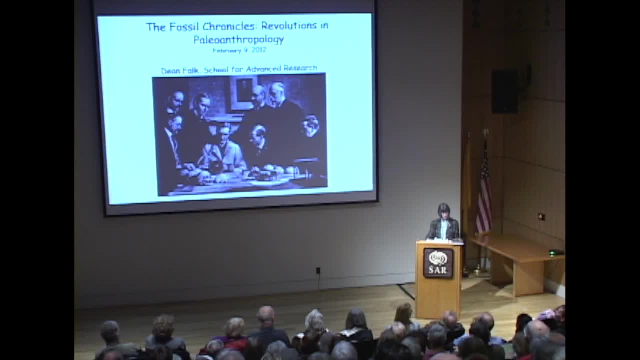 kind of hobbit you would like to hear about, So you could leave now if you had that in mind. I want to talk about two revolutions in paleoanthropology, And then I'm hoping to have a little bit of time to talk about a third one that I haven't written about, but it's just getting. 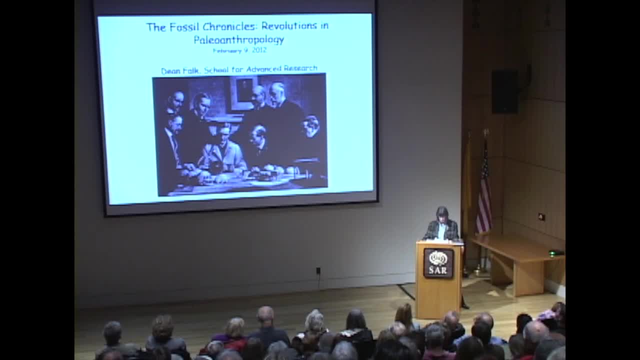 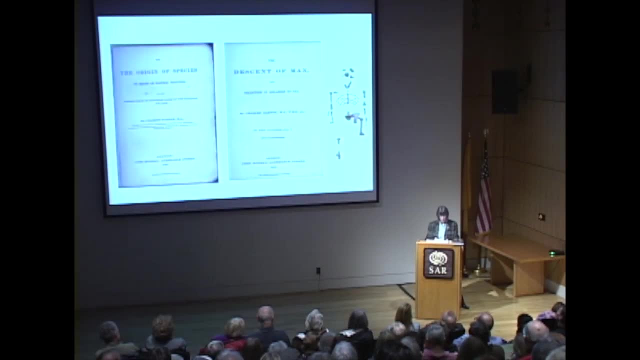 underway and it ties to the first two. The formal study of evolution, as everybody knows, began with Charles Darwin in 1859 when he wrote The Origins. What is not as well known is that he didn't touch the subject of human evolution in that book. He was wary about that because of the 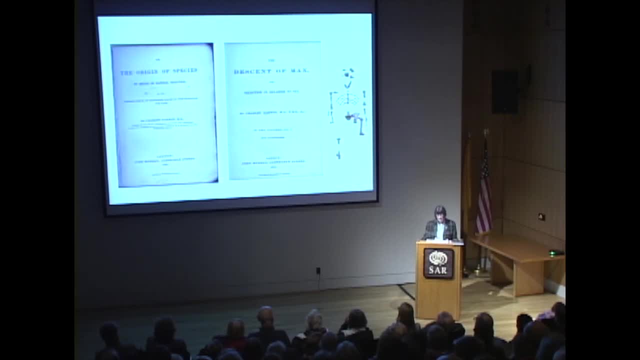 times and because of religious fundamentalism. However, 12 years later, in 1871,, he wrote The Descent of Man and tackled human evolution, And he said that humans are like other animals, They were subject to natural selection. And furthermore, I, Charles Darwin, 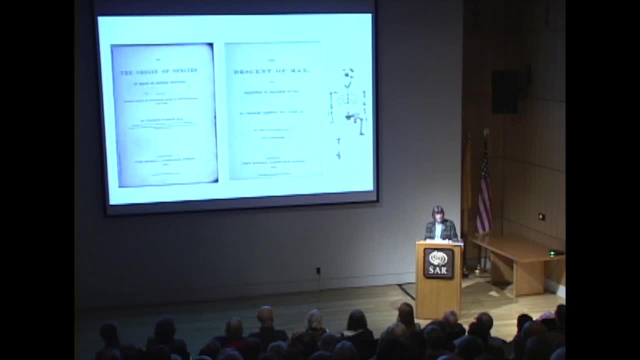 believe that our closest relatives are great apes and, in particular, great apes that lived in Africa, And I think eventually we will find fossils in Africa that are intermediary between apes and humans, And here is one such fossil that has since been found, And he was right, And today, 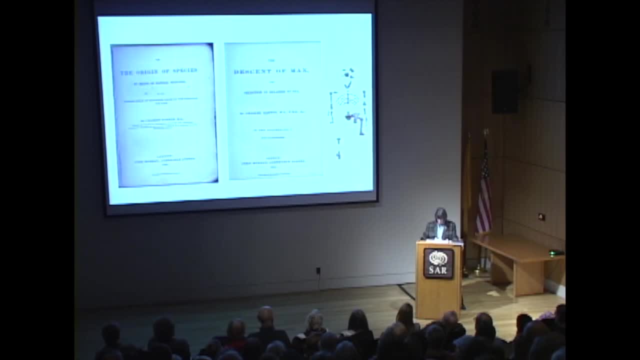 we have a paradigm that was revolutionary then, but it's not now, And this is really where the field's at And it's non-controversial, And so this is the background within which I want to ground tonight's talk. We know today, or there's loads of evidence which suggests that living people and living 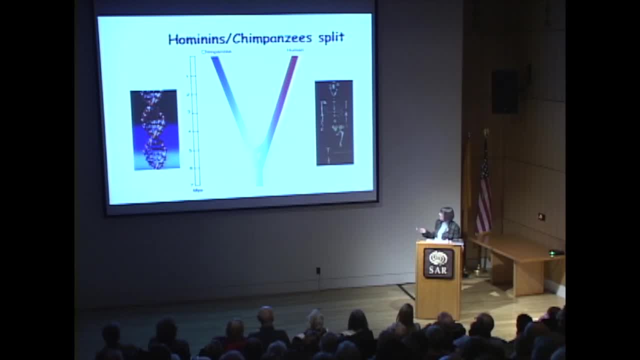 chimpanzees share a common ancestor that lived between five and seven million years ago, And there have been many, many fossils found in Africa and elsewhere which show that Lucy, for instance you've heard of, She's at about 3.2 million years, And there's also comparative genetic evidence from the genes of 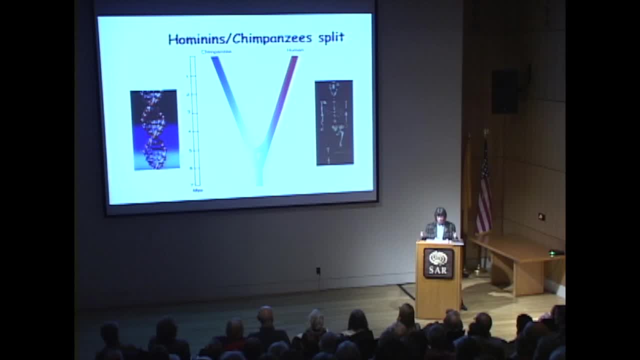 monkeys, apes and humans, which have allowed evolutionary biologists to time these events, And so they're the ones that helped put the date on this. So this is a general paradigm And people sometimes say: oh, evolutionists, they say chimpanzees- are our ancestors, But that's not it. 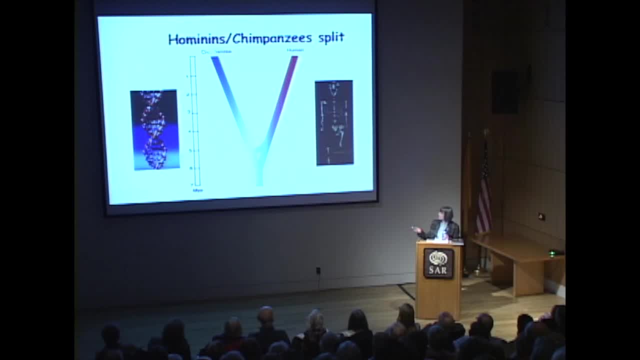 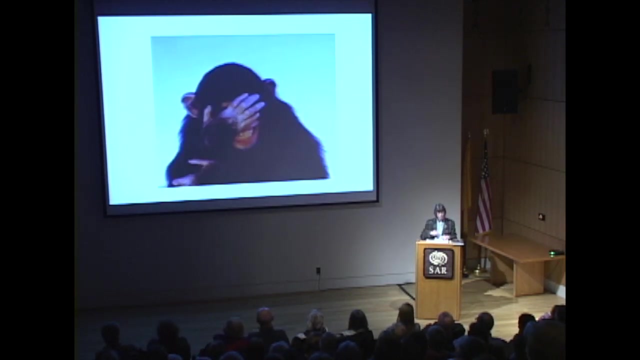 at all. What they say is: they're our cousins. We're not descended from chimps. We share a common ancestor with them. However, just because chimps and humans are cousins is no reason for anyone to be embarrassed. Thank you for laughing. I gave a talk in Italy maybe three months ago and said that: 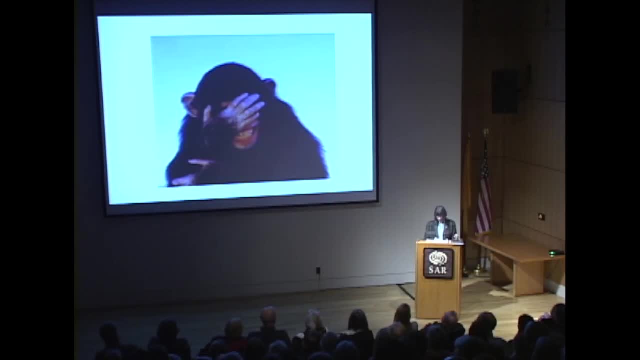 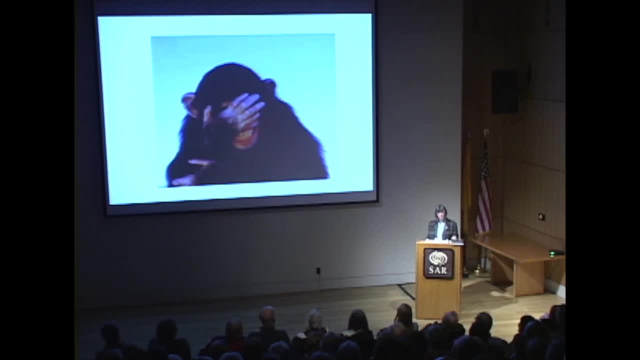 laughing And there was stone silence And I am still trying to figure out why. So I put this in tonight as an experiment In terms of the African origins. though we accept it now, it took a while to get to that revolutionary idea and confirmation of it. For one thing, in 1891, fossils were found. 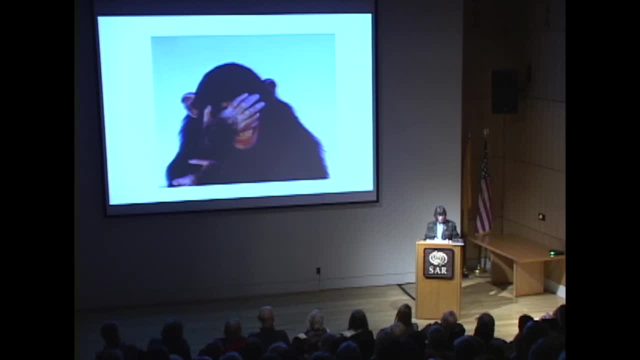 in Java, in Indonesia, which are Homo erectus fossils, And at that time it was thought that our ancestors came from Asia. Another group of paleoanthropologists had a different idea. that developed in 1912. And this is the Piltdown Committee. 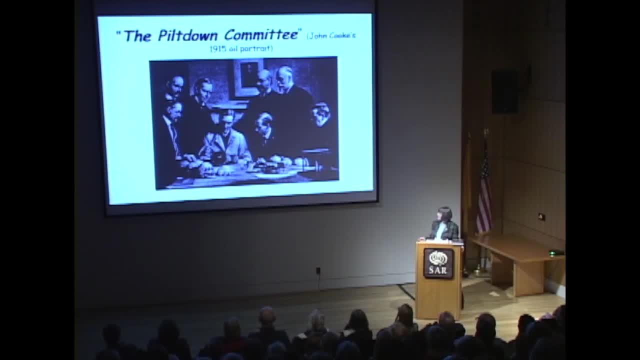 This is John Cook's portrait of them, And they are looking at a skull here of so-called Piltdown Man. This is Charles Dawson, whom I'll speak about in a moment. This is Elliot Grafton Smith. Piltdown was announced at the Geological Society in London in 1912. 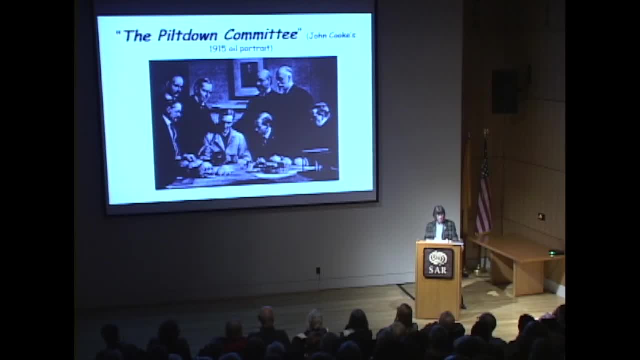 as a discovery of the true ancestor of human beings from England, And the British establishment loved it. They said: ah, the earliest ancestor was a British gentleman, not somebody from Asia like that Pythagorean, That's a Greek Anthropos, that Homo erectus, and certainly not from Africa. 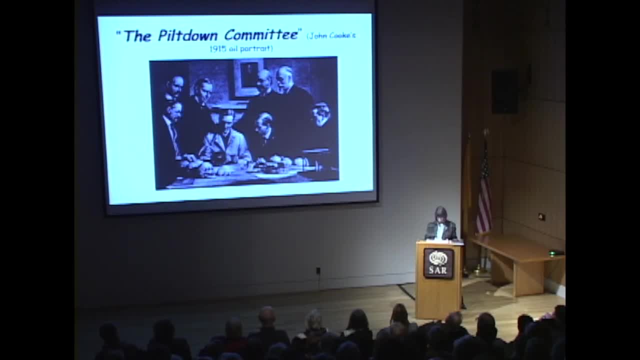 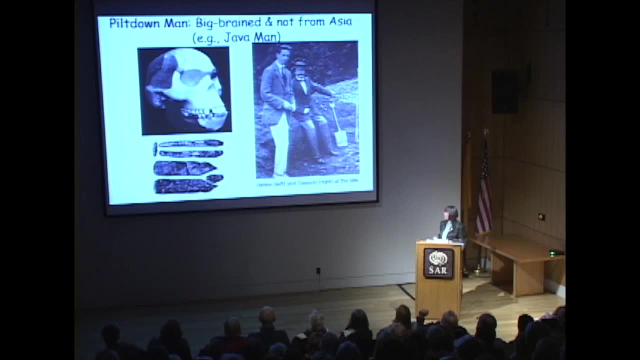 What they didn't realize at the time was that this was a complete forgery, And it was a forgery that held on and had a huge negative influence on paleoanthropology for decades to come. Here is a Piltdown skull. The white parts were missing. 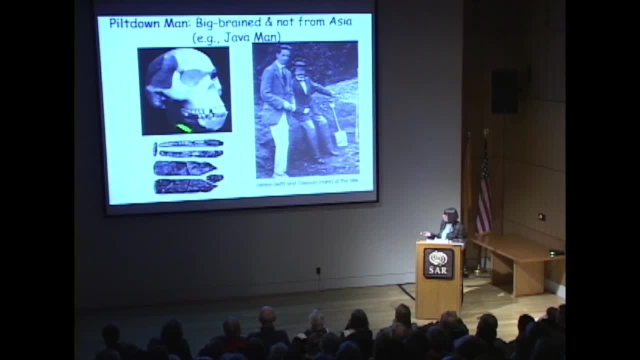 And what it was. it was a human brain case Wetted to an orangutan partial lower jaw. This is missing, this white part and this part back here at the back of the jaw, And it had been stained and the teeth had been filed, so it looked like one specimen. 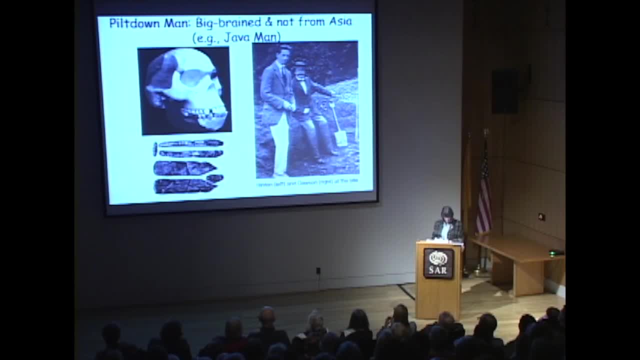 And then it had been salted in these gravel beds at Piltdown in England, along with doctored stone tools and doctored animal ancient animal remains that weren't from that part of the world, And the scientific establishment fell for it and they loved it. 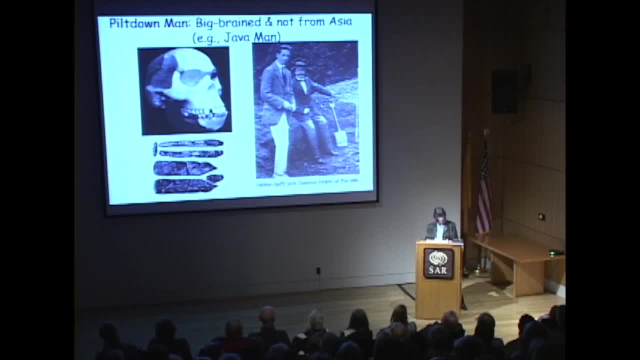 You know, here we are, England, this is where humans originated, And furthermore, it told them that the brain evolved before other things. This is a human brain case. so they thought: ah, the brain led the way. It had a big brain, but in many ways an ape-like jaw, which of course it did. 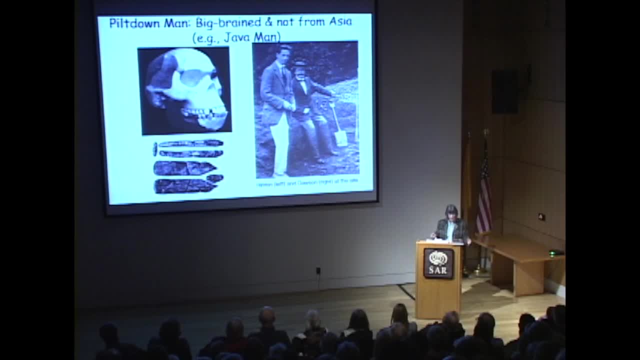 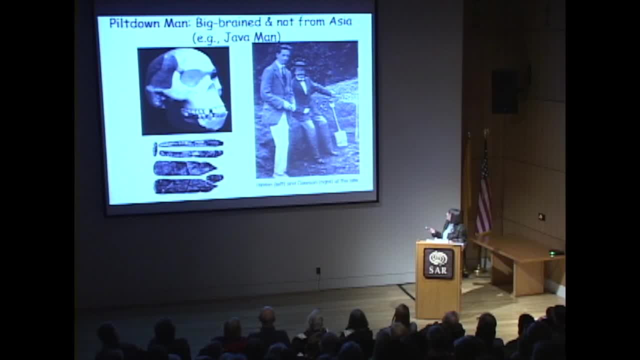 But I think it's now pretty established that Charles Dawson over here, whom you saw in the portrait, was the main perp, But he was aided by a paleontologist. He specialized in rodents, Martin Hinton, And it started out as a practical joke, although Dawson, who was completely unscrupulous, I 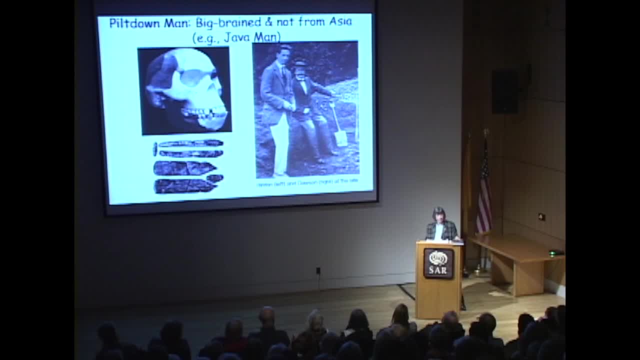 mean he plagiarized two volumes on a castle. He swindled some people out of real estate. He wanted to be in the Royal Society and he used his fine to persuade members to nominate him. So he had a motive, Hinton. 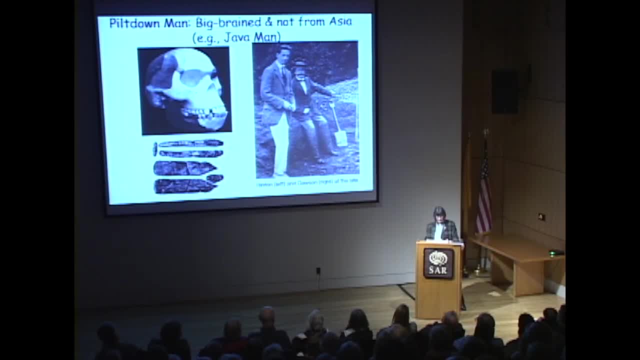 Hinton was known as a practical joker, And as this thing unfolded and they got deeper and deeper, it seems as if they realize this is not good, This is influencing science, And so I think, perhaps to try and make it clear this is a joke, they planted here a. 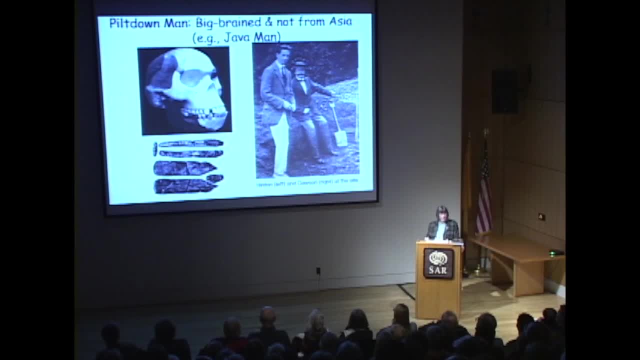 carved elephant bone. you see it in various views that looks suspiciously like an English cricket bat кад주�. And the scientists said, wow a tool. and accepted it as legitimate. So Piltdown Man was believed to be legitimate until 1953,. 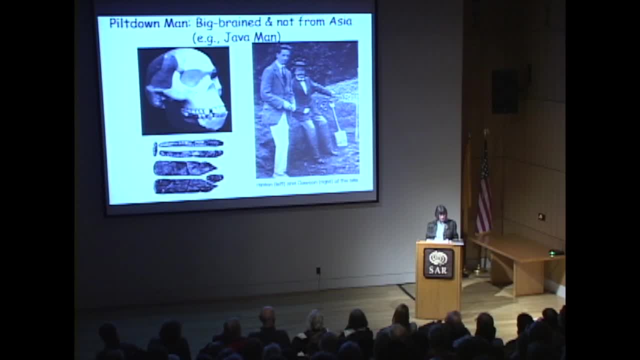 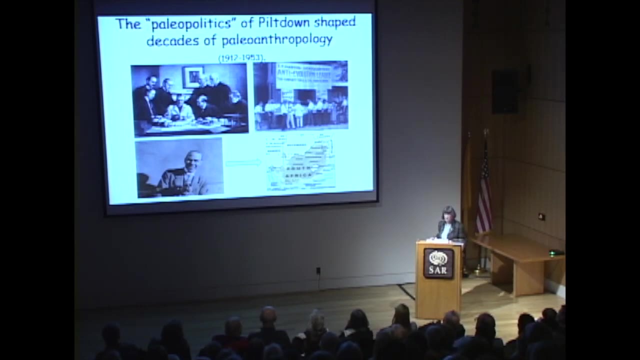 and the luminaries of paleoanthropology in England defended it acrimoniously. They fought with each other, but they basically accepted it as the earliest ancestor. One sees, when you read the literature from that time, what I call paleopolitics. 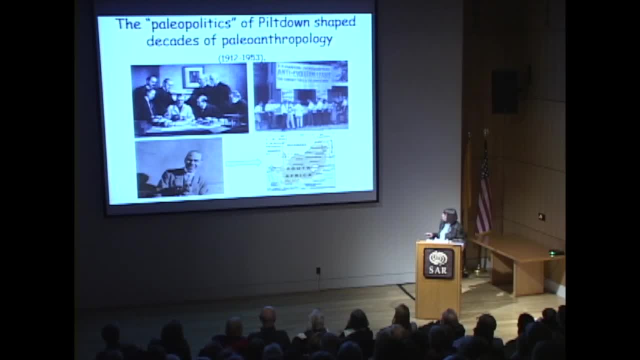 You see, the competition, the digging into published ideas. And they certainly did, and they accepted it, even though they had their differences. It's to me ironic that the only people that figured out early on that this in fact was not real were fundamentalists. 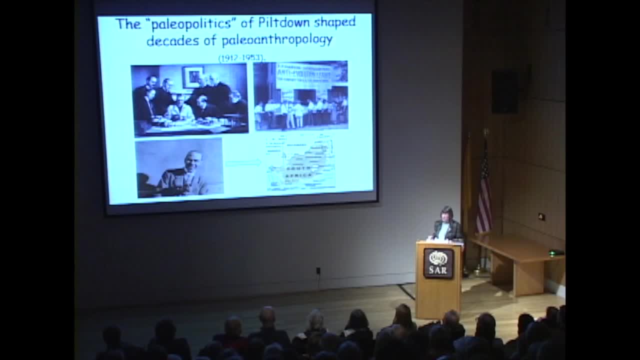 The orator Williams Jennings Bryan, who in 1925 would be the prosecutor in the Scopes Monkey Trial in Dayton, Tennessee, said in 1923, you get, you know, these guys find a few stray teeth in a gravel pit. 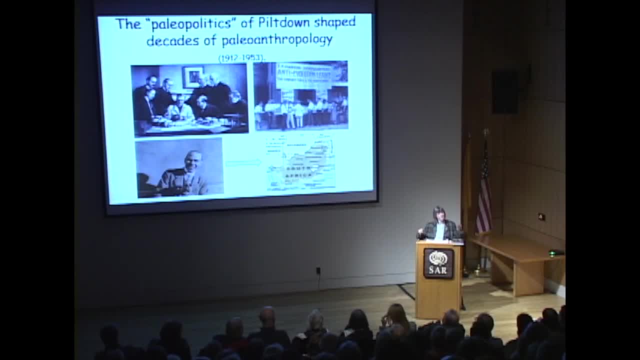 and then they hold a conclave and they conjure up the kind of being that they think you know had those teeth, and they shout derisively: Aunt Moses. So there is that irony. They're always with new finds, are naysayers, religious fundamentalists and scientists. 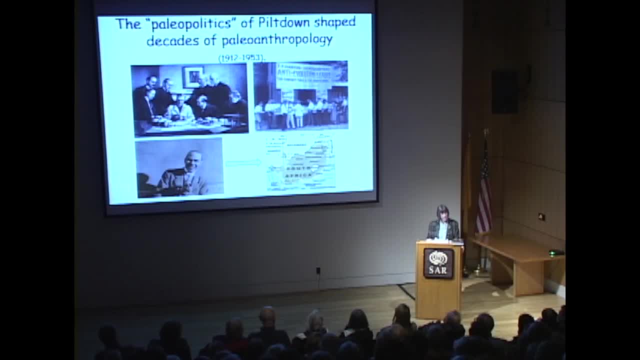 And usually it gets turned around by the discovery of new fossils. But this is the one time where the fundamentalists had it right, and they had it right very early on. But the find was destructive for those scientists who accepted it and devoted their lives to it. 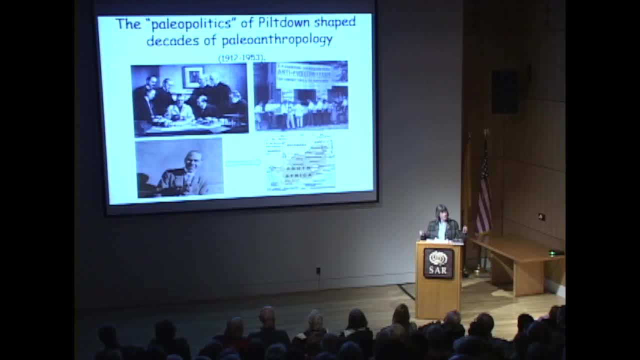 And there's another. There's another sort of irony, which leads me to the first revolution in paleoanthropology that I write about in the Fossil Chronicles. When this was going on, the announcement was 1912, the portrait 1915.. 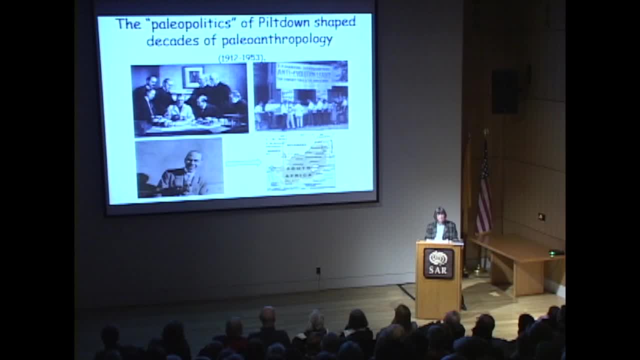 Raymond Arthur Dart, a young Australian, was studying medicine and biology in Australia And he was struggling with his own religious upbringing, which had been fundamentalist because of his keen interest in nature and natural history, And he came to terms with that as a scientist. 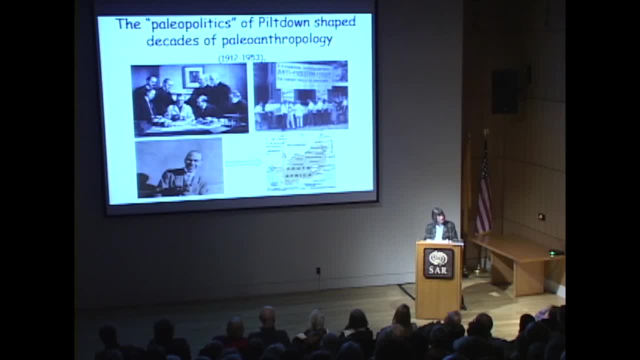 but as one who was highly ethical and kept his moral and ethical standards for the rest of his life. He heard Elliot Grafton Smith, whom I pointed out in the portrait, speak in Australia about brain evolution And Dart said: I want to do that. 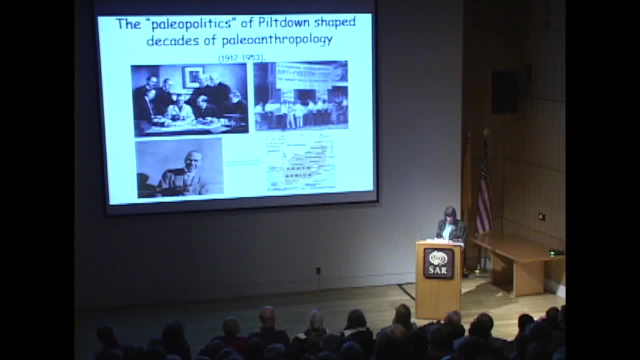 I want to devote my life to studying anthropology and brain evolution. So he got himself shipped. He got himself shipped out to University College London where Grafton Elliot Smith was really establishing the future of paleoanthropology. He was head of the anatomy department there. 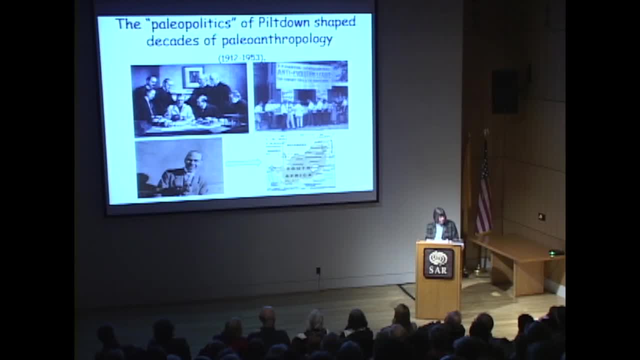 He was training young minds who would go off and make major discoveries. And he took Dart in to teach And Dart thought he was in hog heaven in London because of the collections, the embryological collections, the fossils, the libraries. But in 1922, Grafton Elliot Smith said to him: 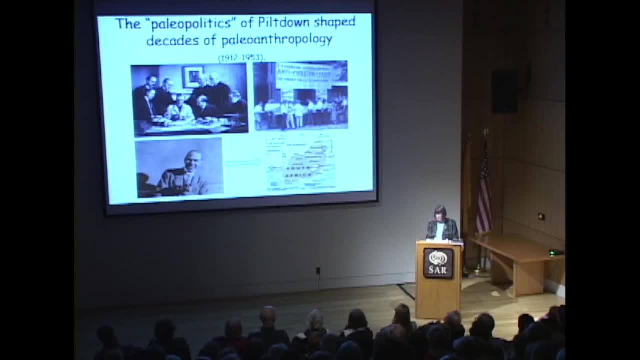 Raymond, there's a position in South Africa at the University of Witsvatersrand. They need somebody, an anatomist, to go down there and build and head up their anatomy department. And he did not want to go. He didn't want to leave this mecca, he was in the scientific mecca. 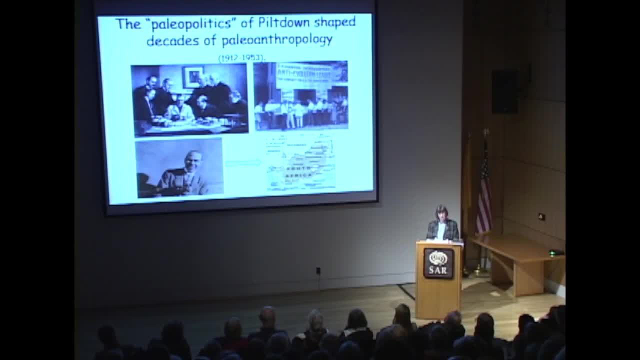 So he tried not to. He tried very hard not to but ended up being sort of guilt-tripped- It's your duty- into going to South Africa. So he set sail with his wife in 1922, near Christmas, and went to Johannesburg, South Africa. 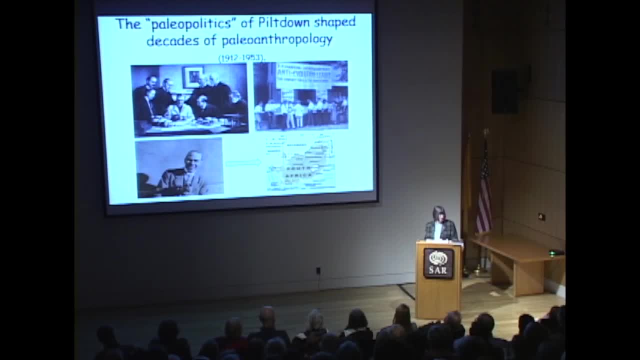 And things were just as bad as he feared. The dissecting room was a mess, There was no library, There were no fossils, But he threw himself into it and began to build what is now a world-famous department, thanks largely to his efforts. 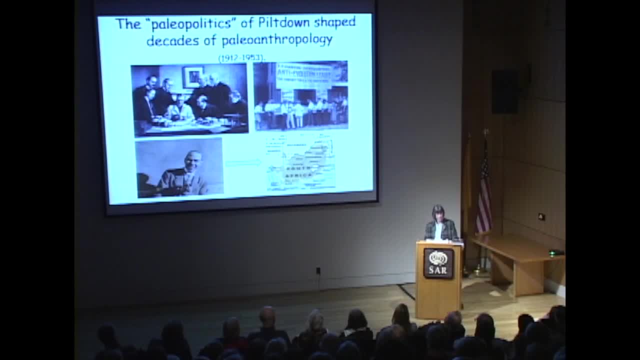 One of the things he did was have a contest for his students, his science students, to bring in the best fossils to build the collection, And because of that he ended up, fairly soon after he got there, in possession of this fossil. 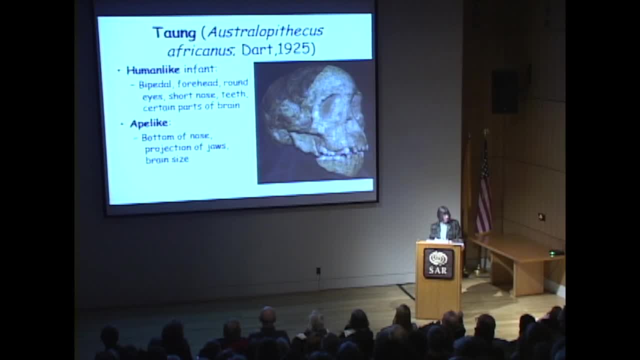 I think this is the most famous fossil in the world. It's called the Tongue Baby and its name is Australopithecus africanus, And Dart spent a couple of months with his wife knitting needles freeing the fossils. It was in two hunks of Brescia. 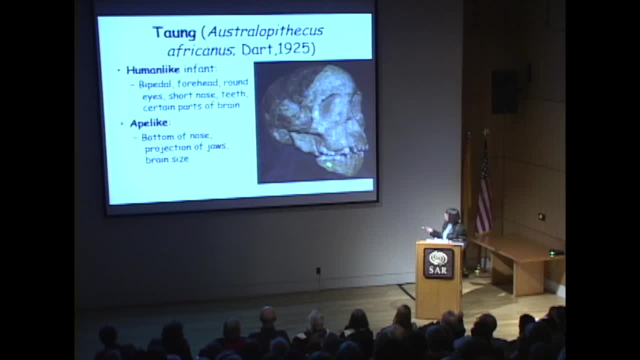 Freeing it and cleaning it off. The lower jaw was still glued to the top jaw And when it got done- at the end of 1924, he realized he had something totally unique in this fossil. It was an infant with, as Darwin had predicted- 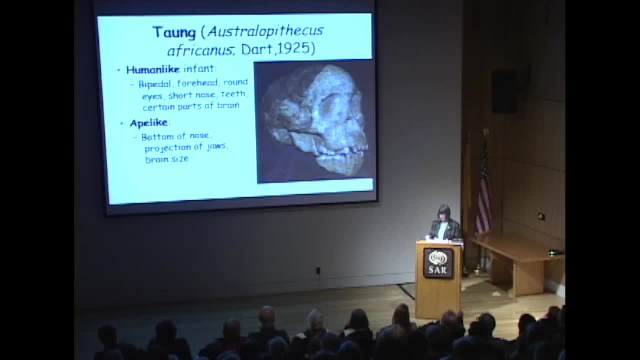 human-like traits and ape-like traits. For instance, it's small, But that forehead, that's not an ape-like trait. And it's not an ape-like brow ridge And the sockets for the eyes are round. Okay, that's human-like also. 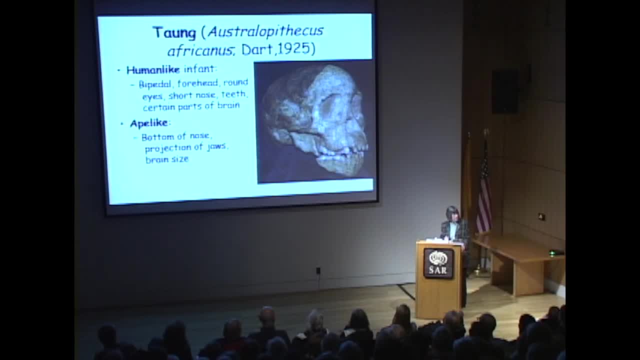 And the nose is short. That's human-like. However, there were some other features that didn't look human-like at all. There's guttering at the bottom of the nose And the jaw region sticks out in front- Totally unhuman-like. 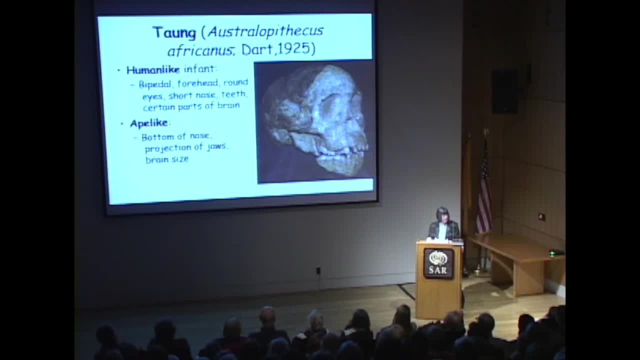 Dart knew that the brain which was ape-like in size. he knew that was an ape-like feature, but he thought he detected a feature on the brain which he could tell about from this part back here. He thought that it looked human-like. 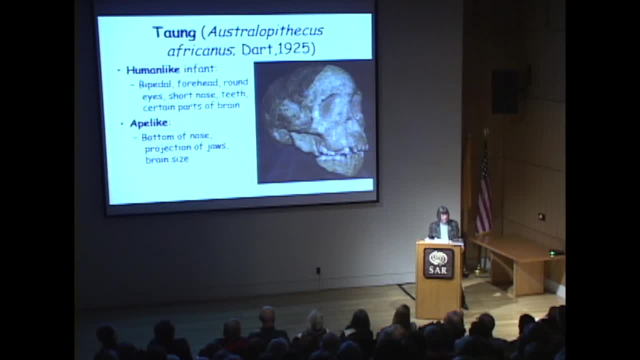 And what this is called is an endocranial cast, or endocast for short. And what happened was, when the infant died, its skull filled up with fine-line sediment that over the years, fossilized. the skull back here disintegrated, leaving this endocranial cast. which reproduced the shape of the brain and features of the cerebral cortex that had been imprinted in the brain cast. So what did he do? It's the end of 1924.. He worked fervently, He wrote up a description, He sent it off by boat to Nature magazine. 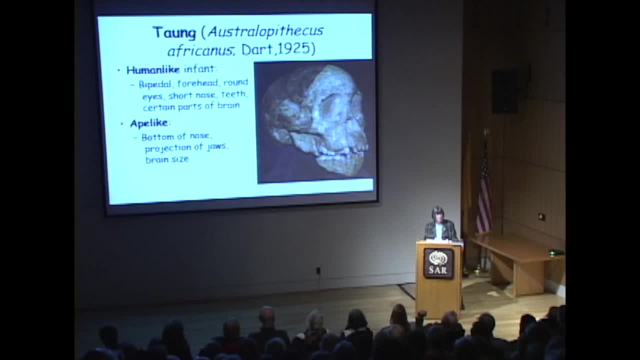 And they were a little wary because the claims were so dramatic. It's a missing link. He didn't use that term, but that's what he was saying, And it's a new genus and species, Australopithecus africanus. 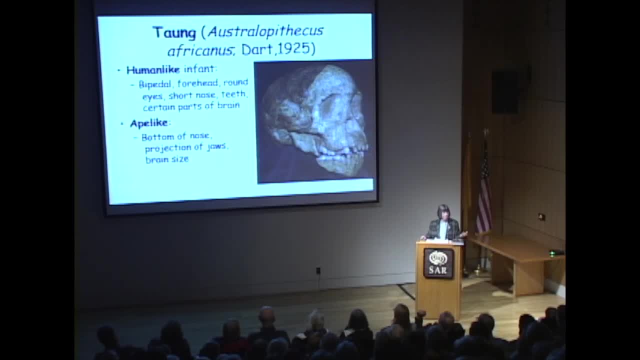 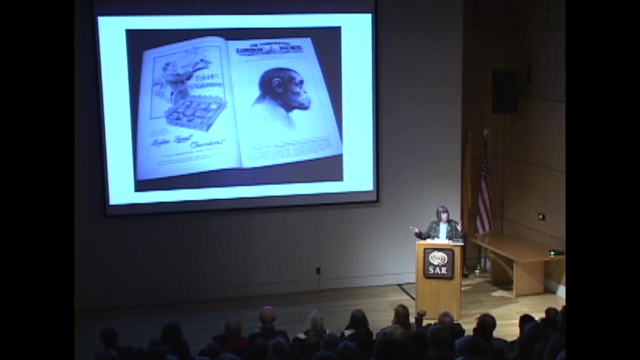 And Darwin was right, This is in Africa. So they had it reviewed and finally it was published on February 7th. Well, he became at age 32, it was like his birthday, February 3rd, which is when there was a leak. 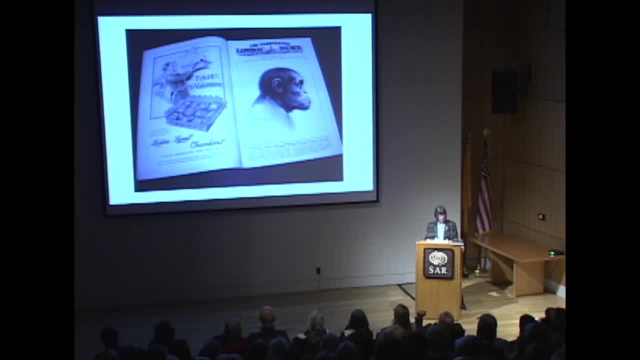 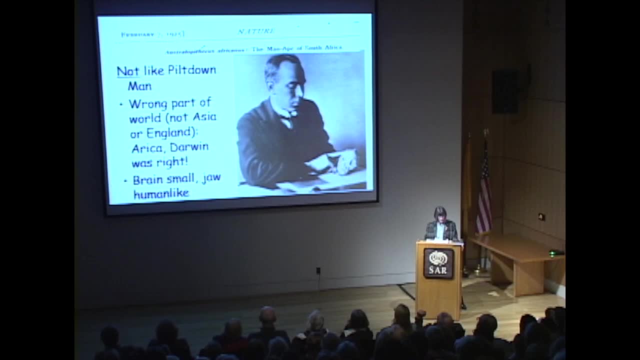 and it became world news overnight. So he enjoyed that for about two weeks until he got the reaction from his buddies in England Because he had said: you know, this is not like Piltdown, It's not in England, It's not in Asia, like Java Man. 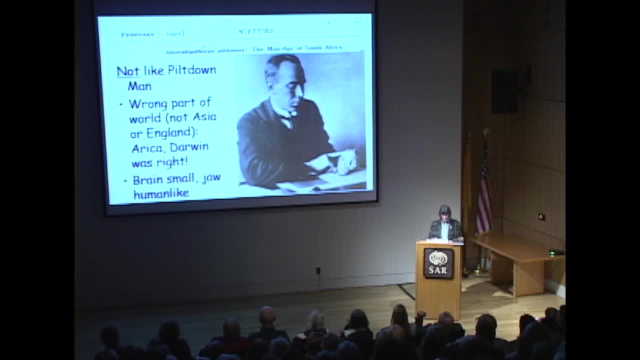 It's in Africa, That's where we evolved. Darwin was right, And he also noted that it didn't have a big brain case or brain like Piltdown- quite the opposite. And it didn't have an ape-like jaw, It had a human-like jaw. 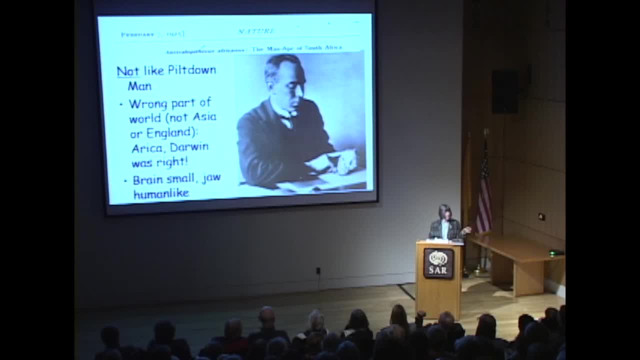 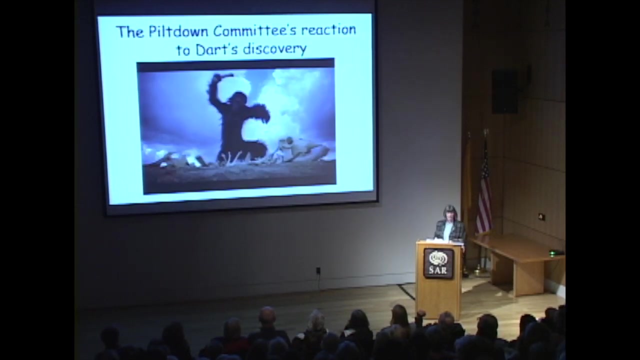 So this was totally the opposite of the expectations. in that day, And here was the reaction. After they congratulated him during the first two weeks and then started writing their own opinion pieces in Nature and elsewhere, here was their reaction: They were not nice. 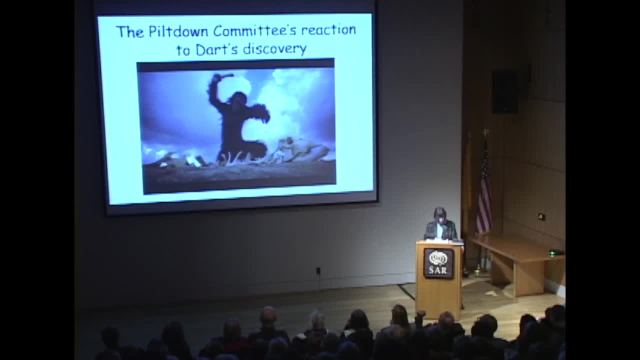 I mean, these were horrible ad hominem interactions. And not only that: Dart, who had been raised as a fundamentalist and retained many of the values, received incredibly vituperative hate mail from fundamentalists telling him he would burn in hell. 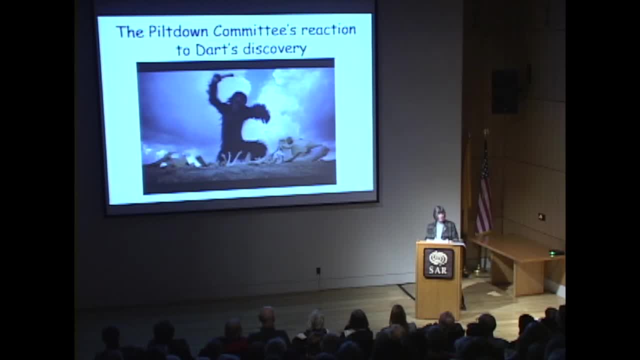 It took a while, quite a while, before his discovery was accepted And I wondered, because of work that my team had done on Hobbit and seeing the horrible paleopolitics and seeing how the politics were actually driving our research and other people's research- 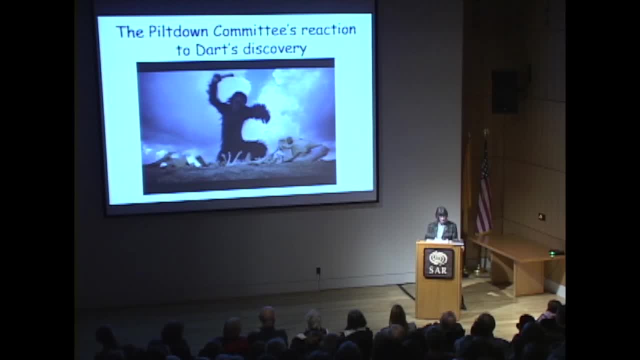 responding to attacks. I wondered you know, how did Dart respond to all these negative opinions he was subjected to for decades? So I went in preparation for my residency here. Thank you, James and Saar. I went in August 2008. 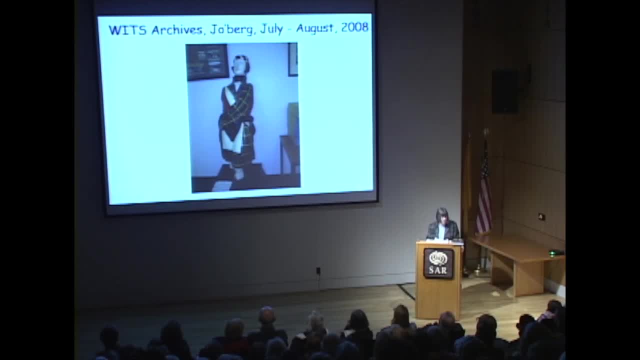 to Johannesburg, to the University of Witwatersrand, archives which had all of Dart's personal papers, which surprised me. I didn't know they even existed and I don't think it was well known at all, But they did and I went there. 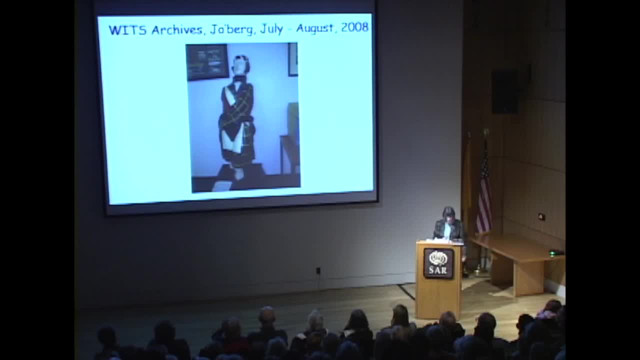 This is Phineas, who used to be the mascot at Witwatersrand And went through a treasure trove of personal correspondence, unpublished manuscripts. I saw how Dart reacted. He became horribly depressed. He quit anthropology. At one point he had a nervous breakdown. 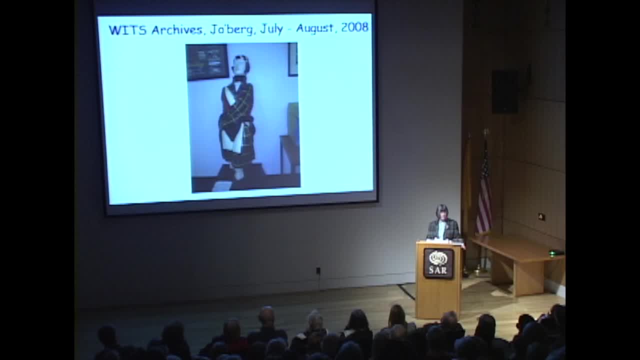 It was a while before his. There were more discoveries of these osteolepithecines, as they're called, and he did turn around. He did go back into paleoanthropology And he was vindicated and his opinions today are accepted. 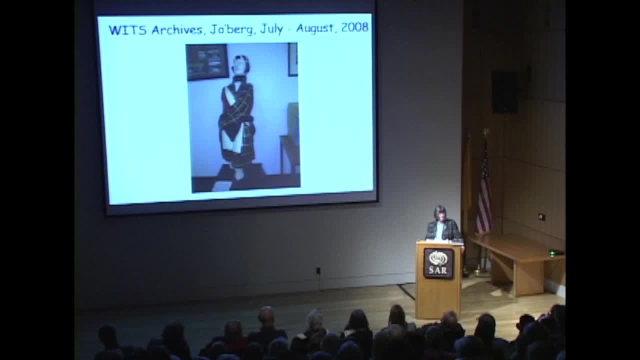 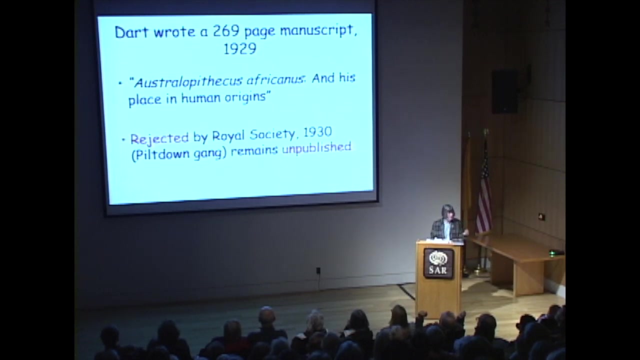 So he died in 1995 at the age of 88, a happy man, But it was tough going. One of the most amazing things in the archives was a 269-page, typed with an onion-skin copy manuscript, And I'm not talking about our pages. 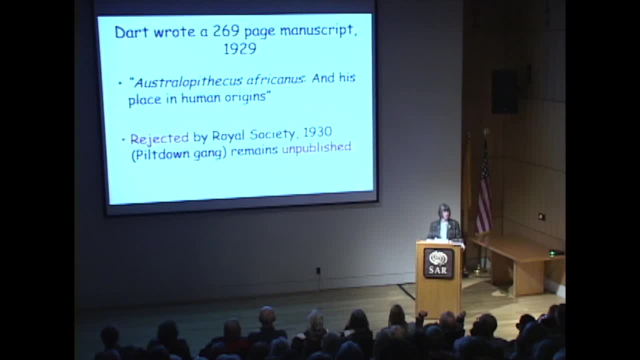 I'm talking about these pages, And he wrote a book on osteolepithecus africanus and his place in human origins, And he'd finished this within four years of his publication in 1929.. And it's rich with the details. 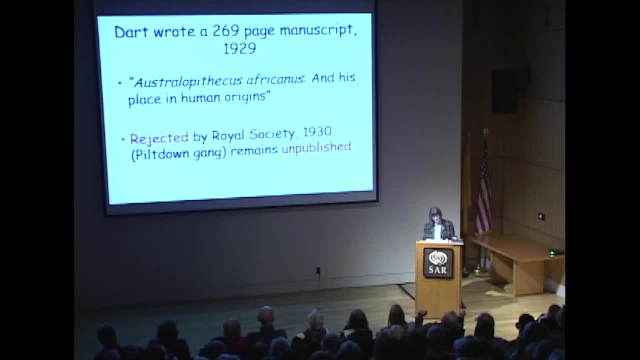 that are not published yet, including what's near and dear to my heart: that endocast- The endocast. in 1925, he identified two grooves that separate convolutions. They're called sulci Well in 1925,. 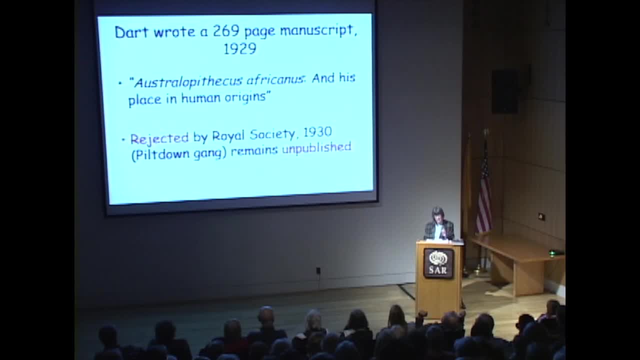 and 1929, he's got 14. And he realized he'd made a mistake. that is important And he had a whole lot about brain evolution. that's sophisticated, and if only had come to light back then. It was actually surprising to me. 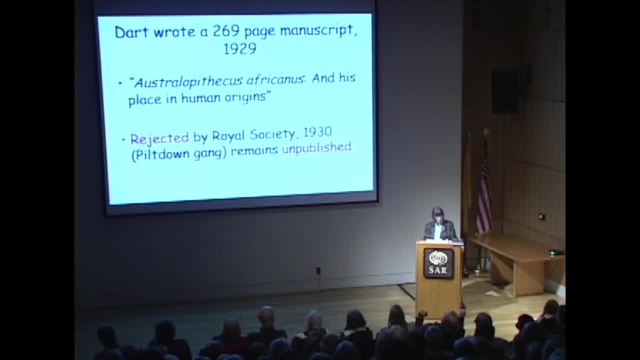 how much functional neuroanatomy was known at that point. However, from looking at this correspondence, it was clear that it was rejected by the Royal Society And it was peer-reviewed by guess who. It was a member of the Piltdown gang who had agreed to present it. 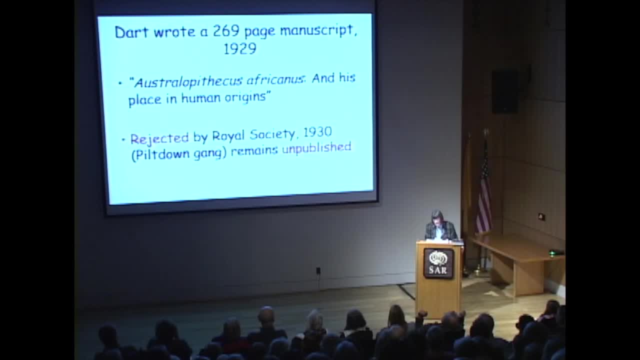 for consideration, And it's a really good bet that those other members, the members of the Piltdown gang that were in the Royal Society, participated in the rejection of this manuscript. I still think it should be published, All right. So from then, 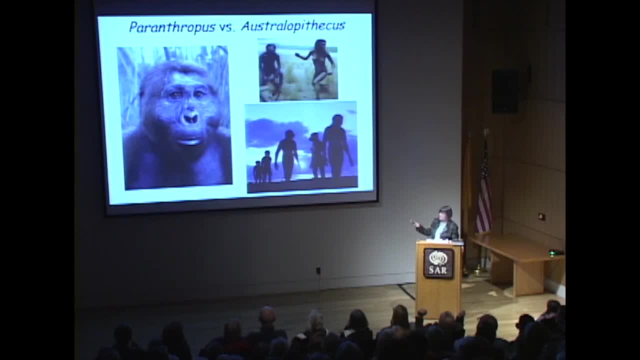 many, many australopithecines have come to light, including in his genus, australopithecus, who may have looked something like this, And a whole other flavor of australopithecine also in Africa. They are all from Africa. 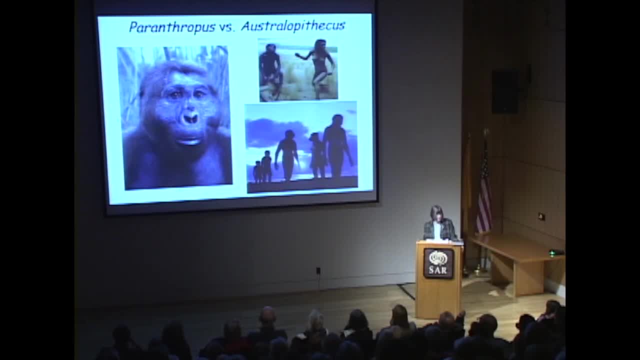 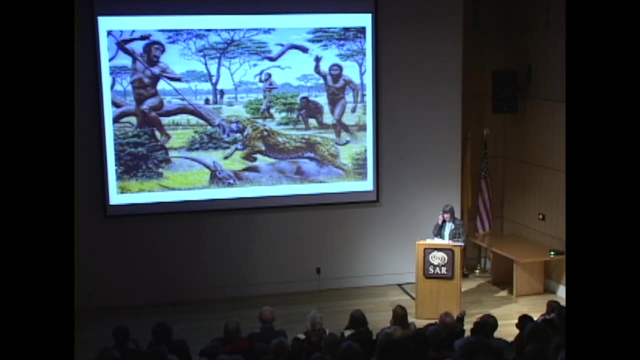 called Paranthropus, who may have looked like that, And Dart was responsible, as responsible as anyone, for a paradigm that had held sway in the literature for a long, long time. You've heard of it: man the hunter. i put this in for george government, who's here, because he has a man the hunter gene. 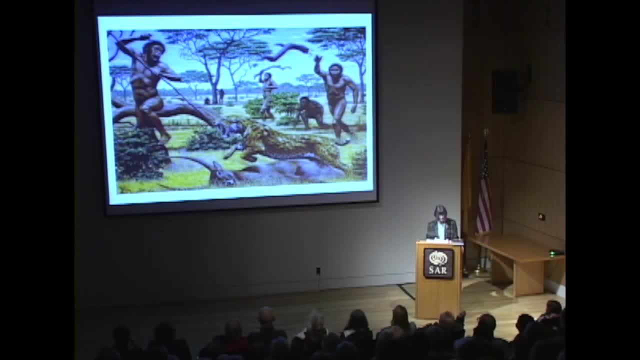 so i thought he'd like to see this, but it was. it was raymond, you know, raymond dart, who really thought a lot, a lot about hunting and and tools and and violence also, and so his find was revolutionary. i think it actually opened up the modern era of paleoanthropology, for one thing. 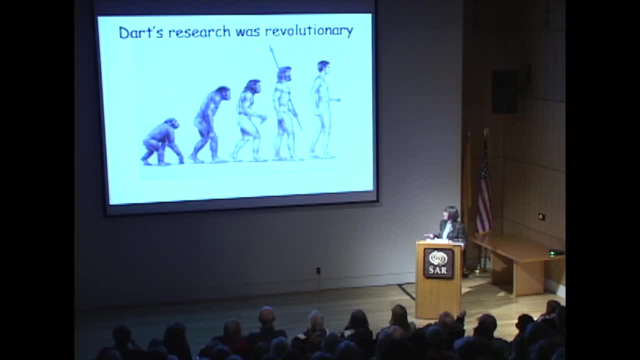 he's showing. you know that that darwin was right- that our earliest relatives originated in africa led ultimately to this idea that we had an african ape-like ancestor at one point, and then eventually, um and osteolepithecine- still all in africa, and then eventually, eventually in this. 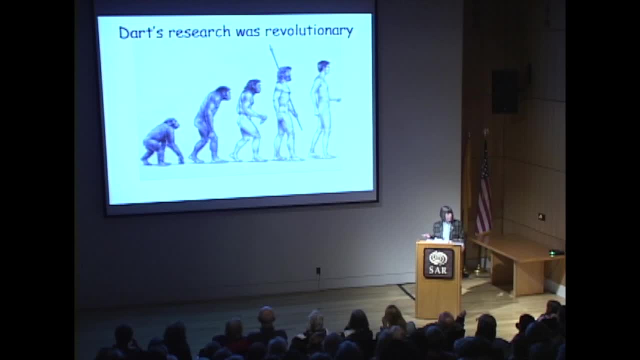 linear kind of thinking: early homo, maybe homo erectus. eventually, who got out of africa? you, you, you And then Homo sapiens, but archaic Homo sapiens And then ta-da, Homo sapiens. So you've all seen this a million times in different kinds of. 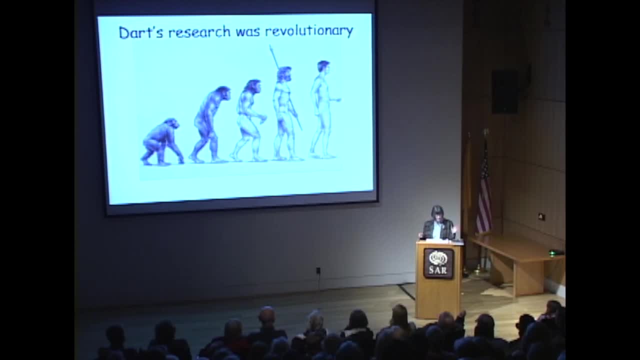 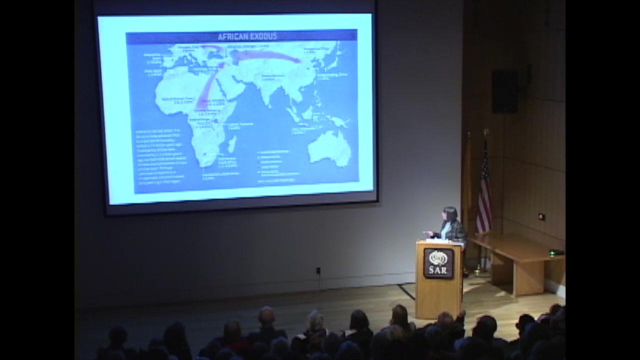 It's used in advertising all the time, And it's this idea of the sequence of more and more evolved ancestors, starting out in Africa, And then- and this stemmed eventually from Dart's revolutionary ideas, and then this paradigm has held sway up until very, very recently. 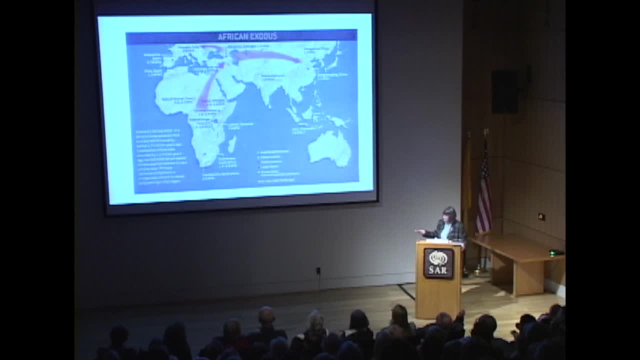 Some people still entertain it that our ancestors split from chimps 5 to 7 million years ago. in Africa evolved the australopithecines evolved, they speciated, there were different species And as we get up near the 2 million year mark, 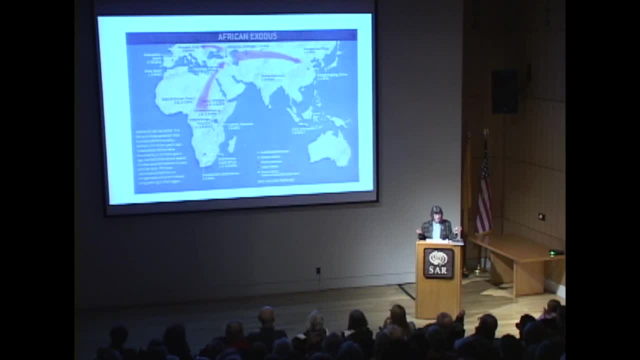 after millions of years of evolution, Homo, early Homo, speciated, And we had from that eventually Homo erectus, who was long-legged and tall, who, about somewhere around 2 million years ago, walked out of Africa and took over the world. 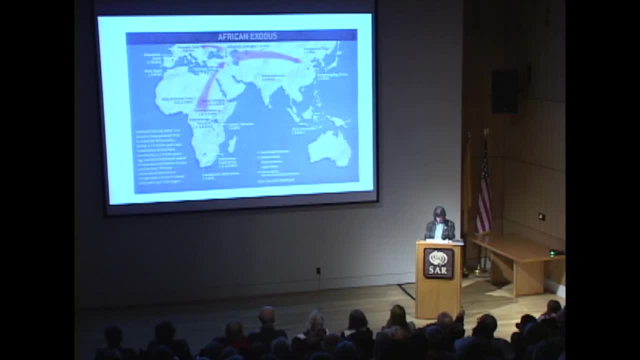 Okay, that's been textbook And we owe the realization that we originated in Africa and that there were australopithecines and that they were important, And that they were important, to Raymond Dart. I want to move to the second revolution. 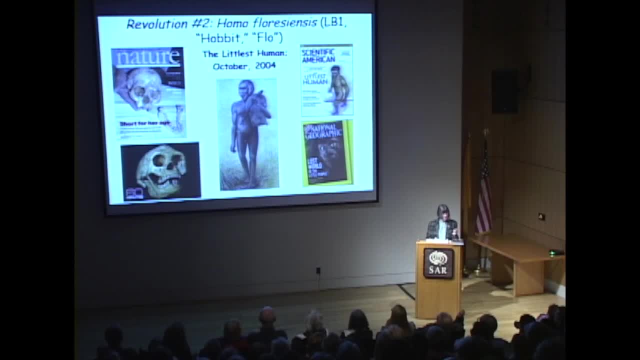 because that's being modified now due to this other discovery. Is this okay, guys? Okay with this kind of hobbit? Okay, In 2004, there was an announcement. Another Australian, Mike Morwood. okay, Arthur Raymond Dart was an Australian. 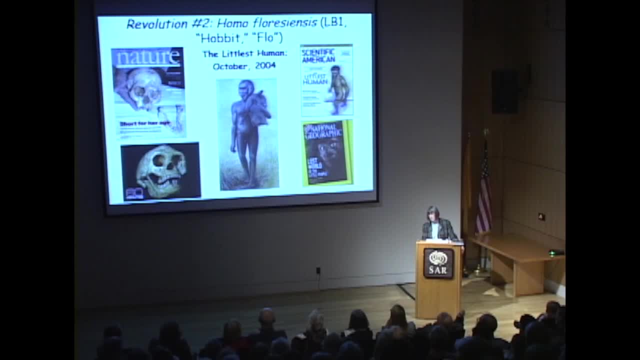 and his colleagues announced the discovery of a new species of human, which they dubbed Homo floresiensis, in Indonesia, on the island of Flores, which is to the east of Java and Bali, And it was shocking. It became world news instantaneously. 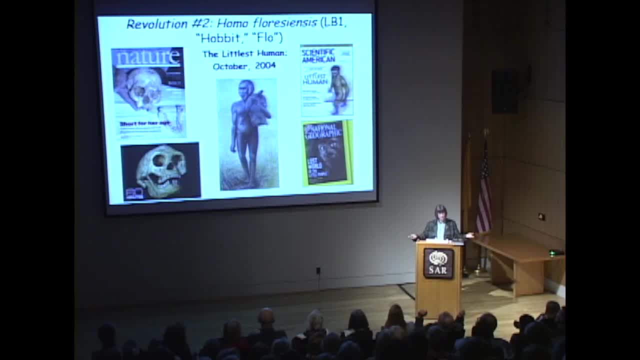 I'd say within an hour of the embargo lifting same journal, Nature magazine, where Tong was announced. It was worldwide news Because the find was so peculiar And again, it was in the wrong place and the wrong time. This picture went out instantly and you've probably all seen it. 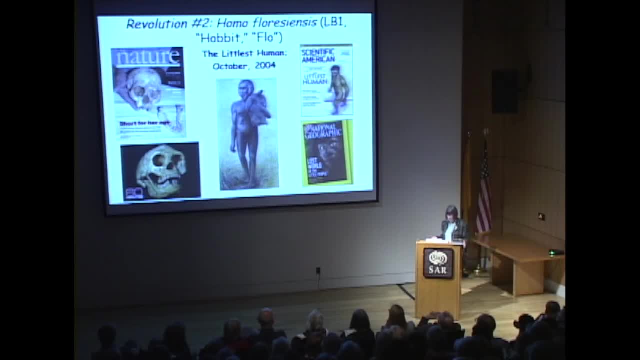 It's the iconic image of Homo floresiensis, who's been nicknamed Flo. There's a problem with this. Flo was a female, but hey, And you can see some of the- you know- immediate media coverage. What was exciting about her was her odd looks. 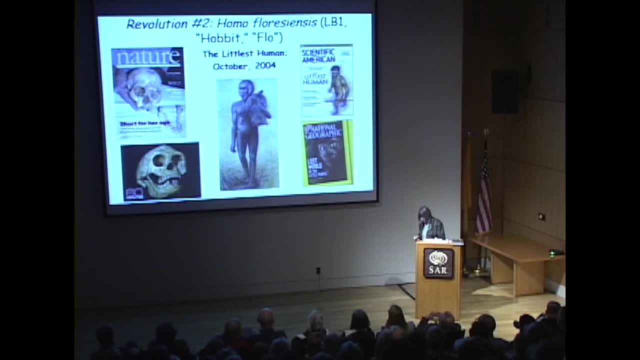 which I'll get into. But also she was an adult female and yet she was at most three and a half feet tall. Now there were fragments of other individuals, maybe eight or nine. She was only 18,000 years old. 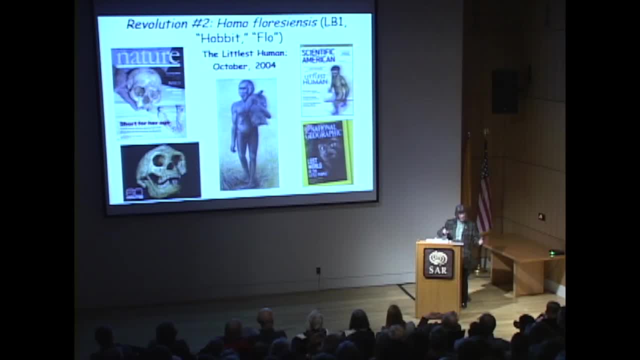 That's nothing. That's yesterday, But these other fragments went back to 95,000 years ago and they resembled her. Whatever part of the body it was looked just like her. She was a big one, three and a half feet tall. 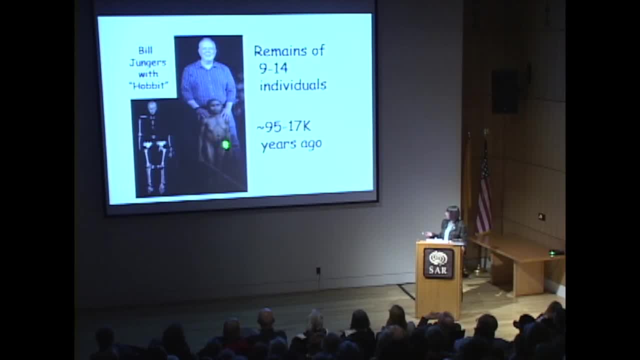 Here's a picture of Flo as a female, which she was next to paleoanthropologist Bill Jungers, who's at Stony Brook, and he's done some of the most important work on this skeleton And, as I said, there are other remains back to 95,000 years ago. 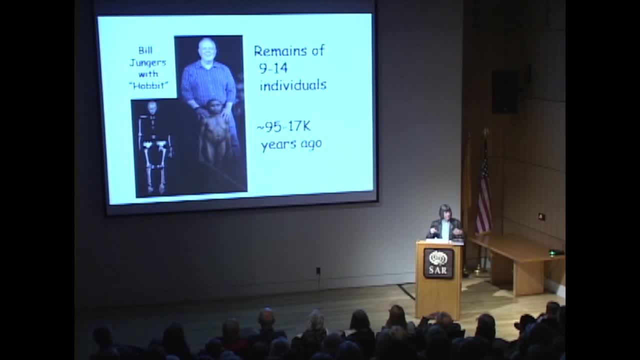 And the estimates, as I said, to how many individuals varies with the workers, But there was a big handful and for instance, there was a little jaw that looked just like her very strange jaw exactly, except it was smaller. 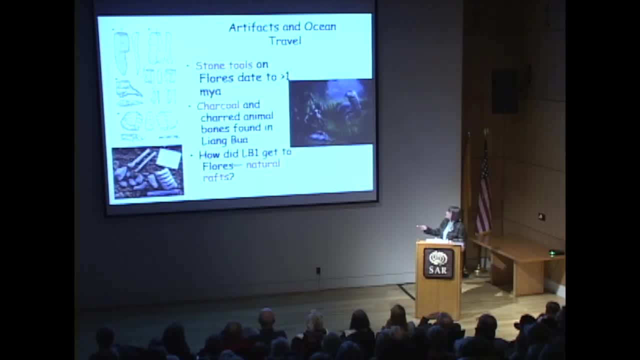 In addition, there were tools in the cave. These finds are all from the cave Leon Bua on Flores And they look like this and these look a whole lot like australopithecine early tools, the earliest ones in the record. 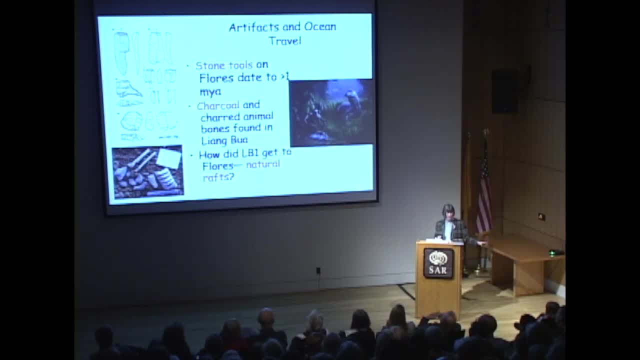 And they are over 3 million years old and they are in Africa. There was indication of cooking or fireplaces in the cave. Flores is hard to get to. There are deep sea currents that make it difficult to colonize, And so the animal life that's there. 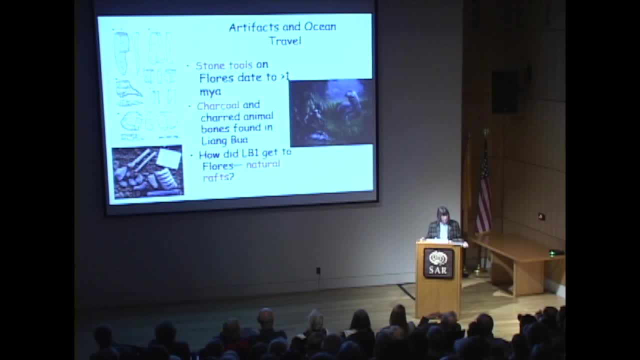 has been there a long time. There's deep time there. You don't have colonization and recolonization. There are giant Komodo lizards or Komodo dragons and there are miniature elephant-like creatures, So some animals got small on the island. 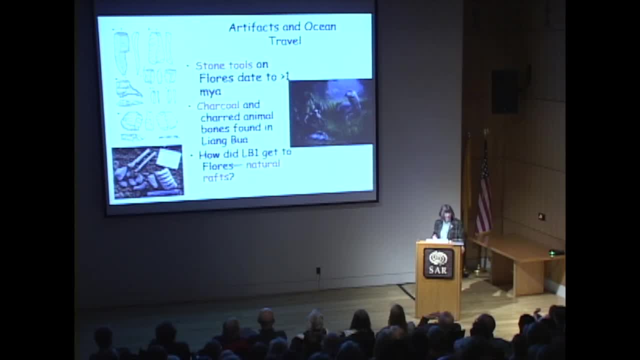 and some got big. So there's a question: How did she get there, she and her kind? The tools are at least a million years old and the remains go back so far to only about 100,000 years ago. And who were her ancestors? 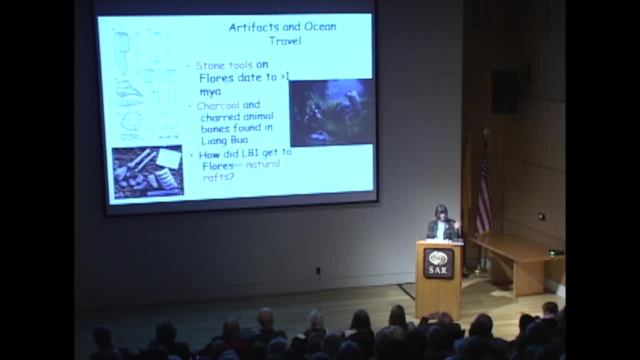 And I'll tell you in a little bit where the field's at. But I want to just mention the research that I was extremely fortunate to be invited to do on this specimen, And it was a surprise to me. They kept the embargo at nature for a year. 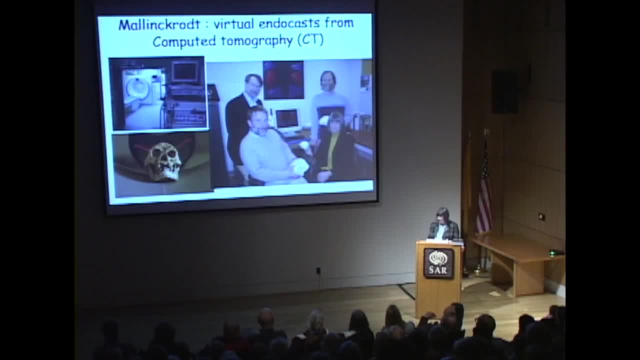 Usually I hear, or often I hear through the grapevine- when something's going to happen. But they really kept this bottled up And at first I was incredulous: What are you telling me? But no, it turned out to be real. 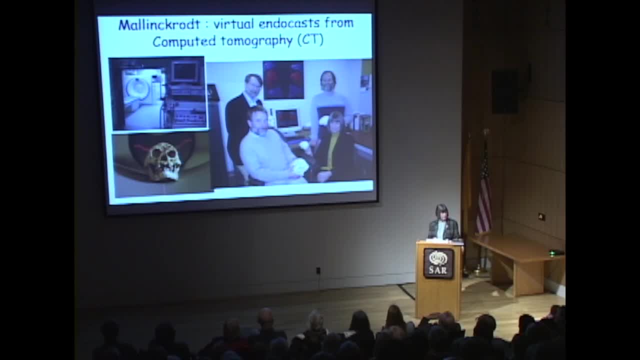 So I was invited to study the endocast and was thrilled to have that privilege And I lobbied and I lobbied hard to be able to do it right, And that meant not pouring liquid latex into a copy of the skull. 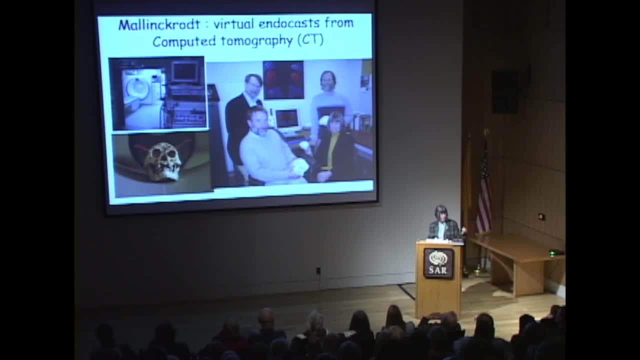 I needed the CAT scan data. It's like a fancy X-ray that would really show details. Mike Morwood, the discoverer, was persuaded to send raw data and CAT scan data to my dear colleagues at Mallinckrodt Institute of Radiology. 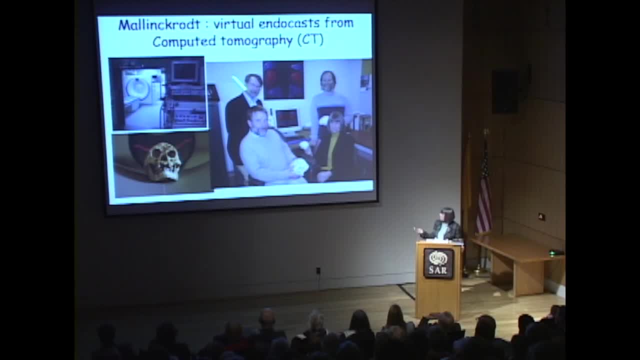 in St Louis, And this is Fred Pryor. It's his electronic radiology lab where we did the work. This is Kirk Smith, a crackerjack engineer, and my buddy Charles aka Scooter Hildeboot, So we took this on. 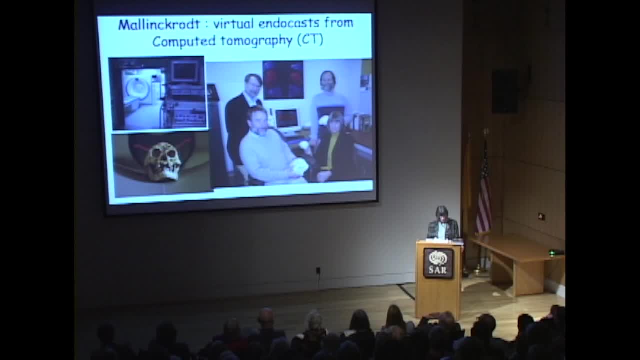 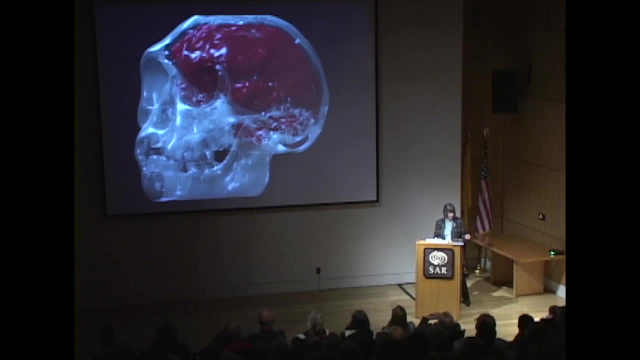 and described the endocast, And I'm going to show you a marvel of engineering. This was rendered by two engineers working independently to check on them, But you're looking at a virtual skull of LB1. And we flood-filled the brain case. 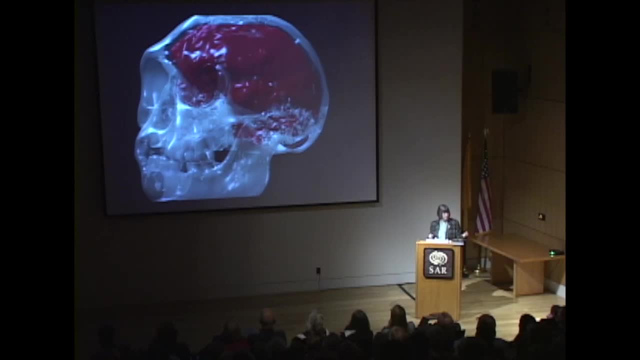 and there is a virtual endocast that reproduces the shape and some of the details of the brain, And these are very nice because you can go, like, into the depths of the bone And you can measure these in ways you can't. 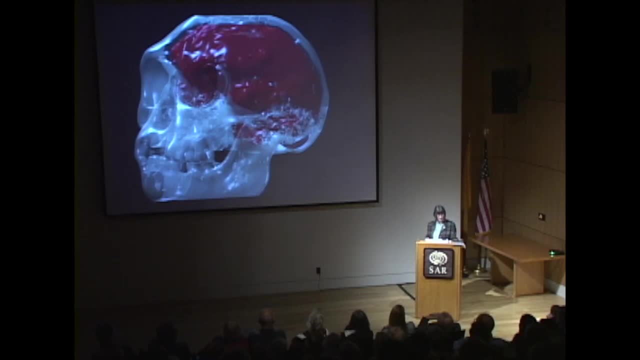 with just physical solids. These are solid endocasts. You can twirl them and dice them and take really precise, really repeatable measurements and keep them within a frame. That's very, very important for doing that. What we discovered, to my relief and my surprise. 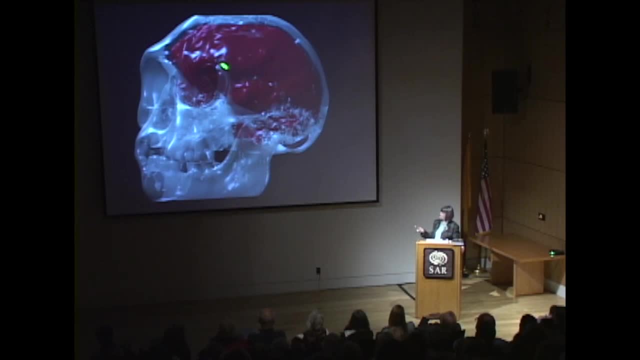 because I thought, oh brother, this thing is, you know, it's only 417 cubic centimeters. That's the size of a chimp brain, A third to a fourth the size of a human brain. I thought Morwood was not going to be happy with us. 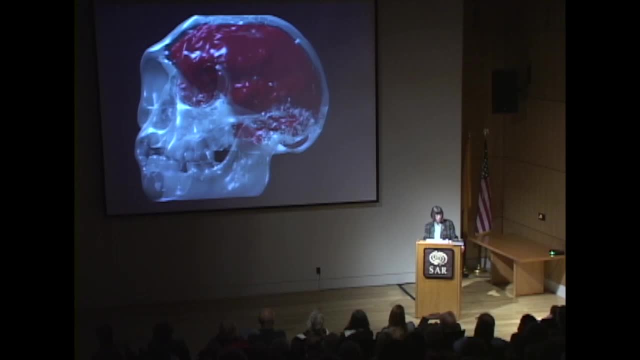 We're going to find this thing looks like a chimp, But it didn't. It's extraordinarily advanced, this endocast, And it's all over. It's from front to back. There are advanced or derived features which convinced us that the discoverers 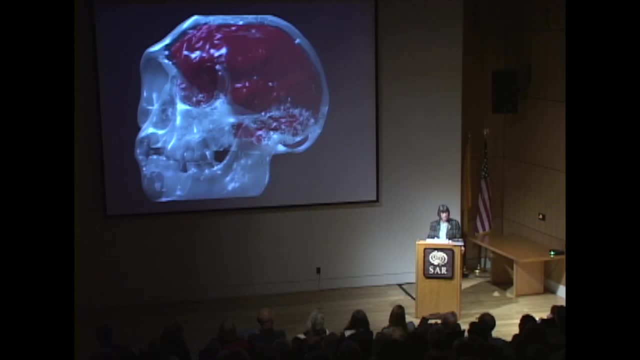 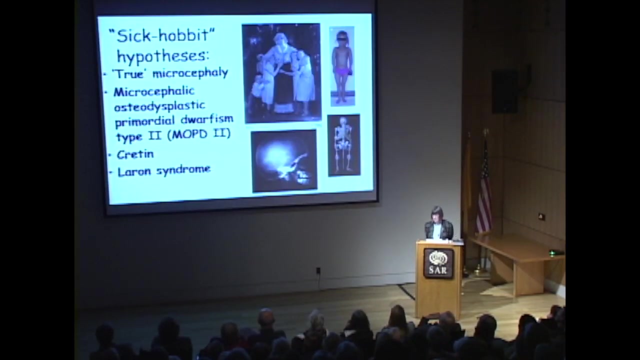 were right to name a new species and to attribute to it the production of the tools they found in association with it, and the hunting and the cooking technology. One of the things we had to deal with were the naysayers. This happens all the time. 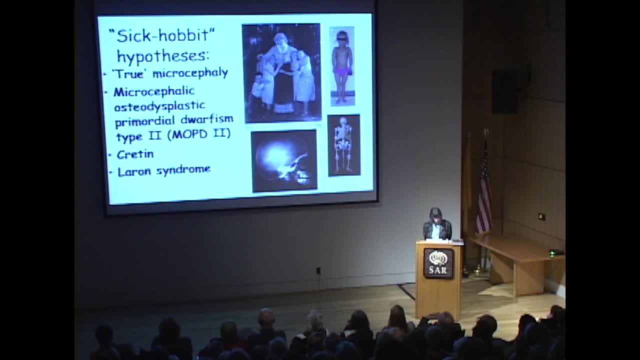 The moment it was announced in 2004,, a small, vociferous group of scientists were all over the discoverers saying: that's not a new human species, You've got a sick human being. Jungers has dubbed these sick hobbit hypotheses. 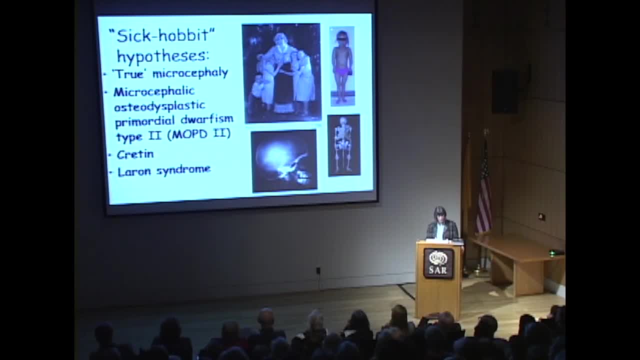 And our brain work, our endocast work, also received treatment from the same group of people And they said: no, That's not a brain of a new species, That's a brain of a human being, Homo sapiens, who has a condition. 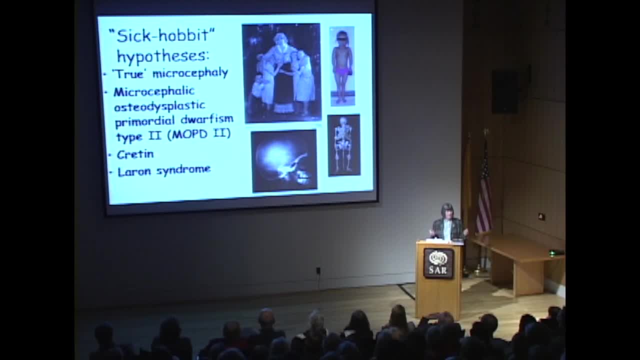 called microcephaly, meaning small head, And you have here a picture from one of my favorite kind of cult movies: Freaks 1932, Todd Browning, with some very famous carnival performers, Jenny Lee and Elvira Snow. 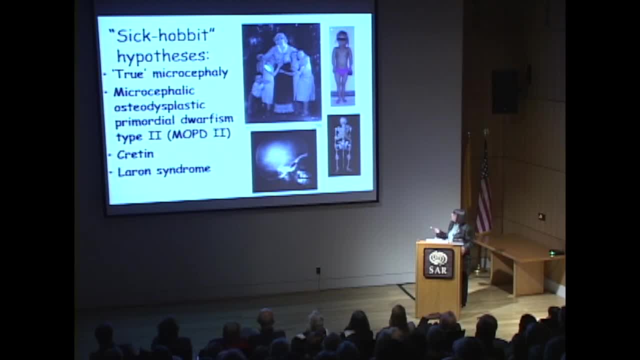 otherwise known as Zip and Pip and Schlitzie, and they're all microcephalics And you can see they have very small heads and kind of pointed. That's where Zippy, the Pinhead the comic came from- is actually some of these. 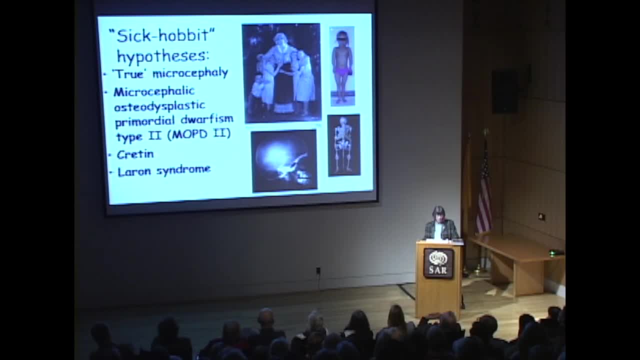 early performers. Because of this criticism, my team had to drop everything- because you can't ignore it- and start studying microcephaly, which turned out to be fascinating. So we did that and did a study, through a thorough study, And microcephaly then went into disfavor. 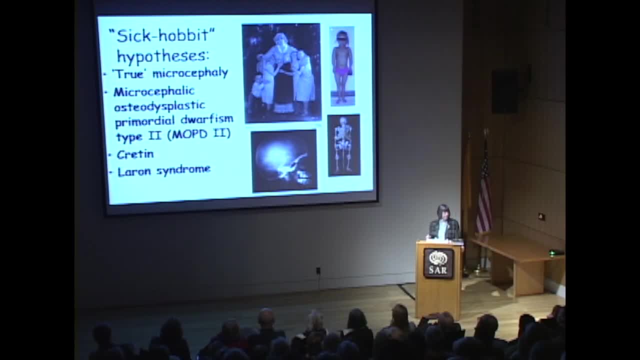 as an explanation. So another kind of microcephaly was proposed, and that was refuted. And then something called Laron syndrome was proposed, And again we had to drop everything and deal with it and did, And that was refuted, And then they went. 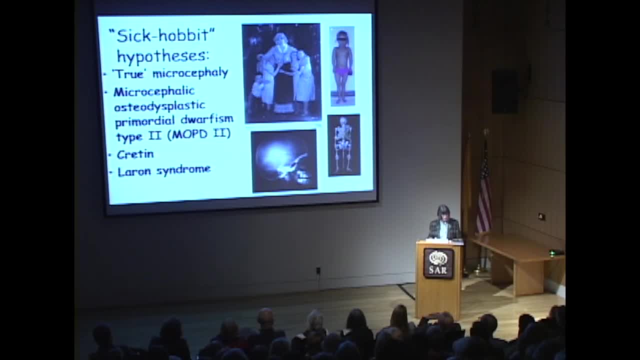 well, it's a cretin. Okay, Peter Brown has something that should be out now in Journal of Human Evolution that just syncs that. So no one to date has come up with one specimen of a human being with a known pathology that looks anything like. 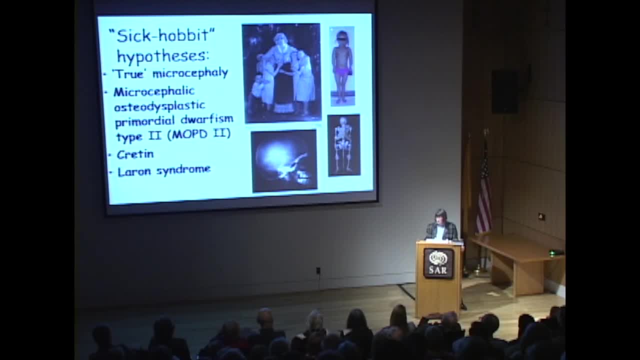 Homo floresiensis. If they do, we're cooked, Because the hypothesis that Homo floresiensis is a legitimate new species is falsifiable And for something to be subject to the scientific method, it has to be: Find us a for sure human being. 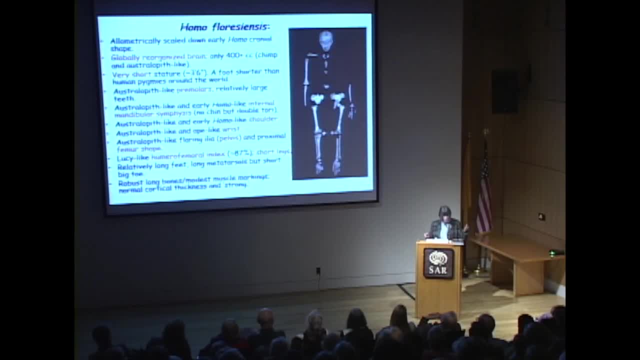 that looks like Hobbit, and you know that would go a long ways towards just syncing the whole idea. this is a new species. Now I apologize for this complicated slide And I'll just say that here is LB1, Hobbit's skeleton. 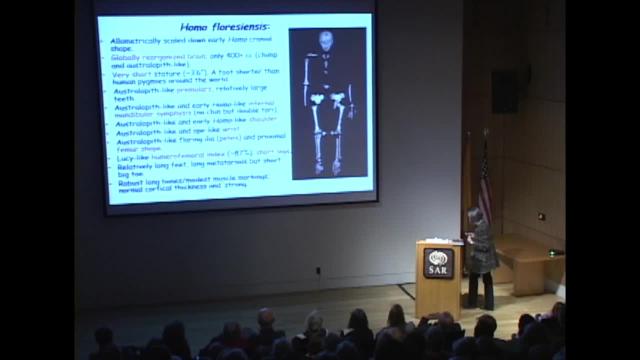 It's pretty complete And different scientists have worked on different parts of the body And what's been found, if you go from head to toe, is that you see features that you see in many other species at different times of the year. So you know. 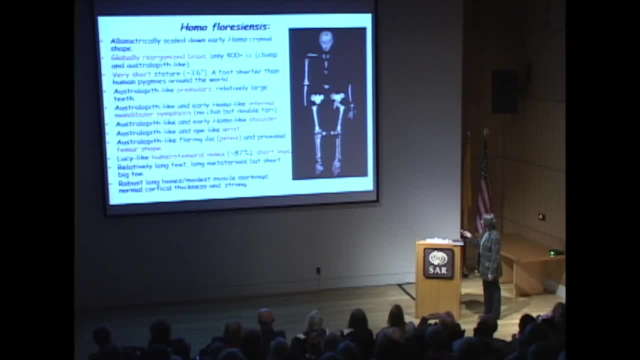 if you go from head to toe, you see features that you don't see in the fossil record, But nothing. nothing looks like this. This is a small skull which in some ways looks like Homo erectus skulls, But in some ways. 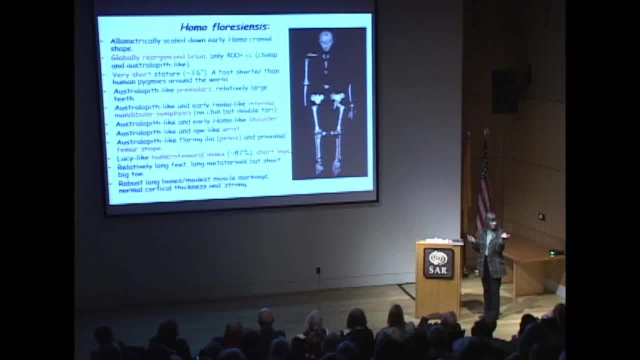 you know, the jaws and teeth look like australopithecines, So it's unique. The shoulder is relatively primitive, The wrists look ape-like, The pelvis. this pelvis looks just like Lucy's. She's an australopithecine. 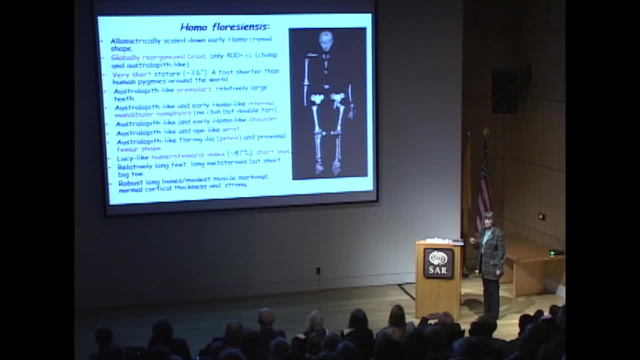 who lived in Africa three or four years ago. So it looks just like Lucy's. She's an australopithecine who lived in Africa three or four years ago and who lived in Africa 3.2 million years ago. The arms are really long. 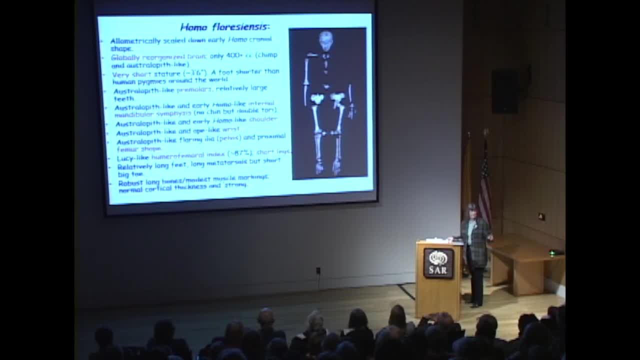 compared to these short little legs And to me the most curious feature is this is a biped. This individual walked on two legs, But the toe was kind of short and the other toe, the big toe, was short and the other toes were long. 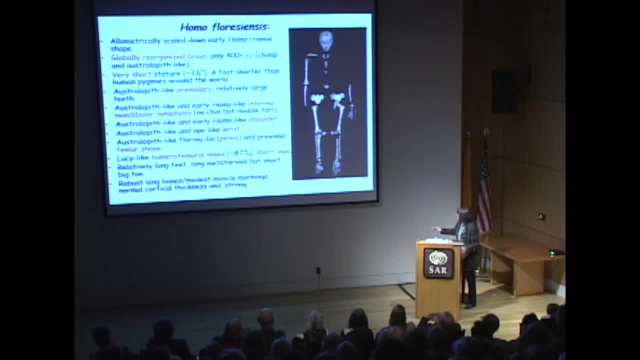 But to me, the most extraordinary feature is that this foot length is the length from the knee to the toe to the ankle. Think about it If you had feet that were that long. Well, homo floresiensis did So. this is something unique. 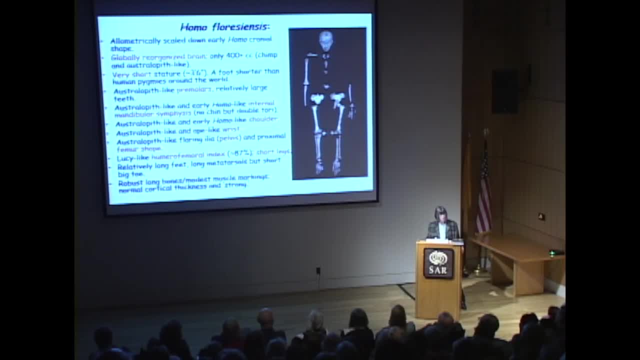 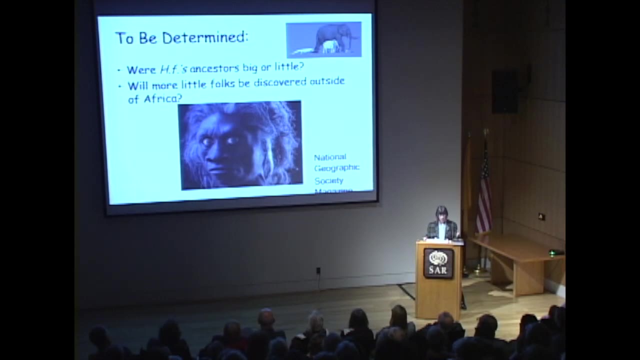 It looks from the tools that its ancestors got to Flores over a million years ago and then it did its own thing. It evolved in its own direction. Okay, People are continuing to work on it. The discussion now is where its ancestors, big or little, 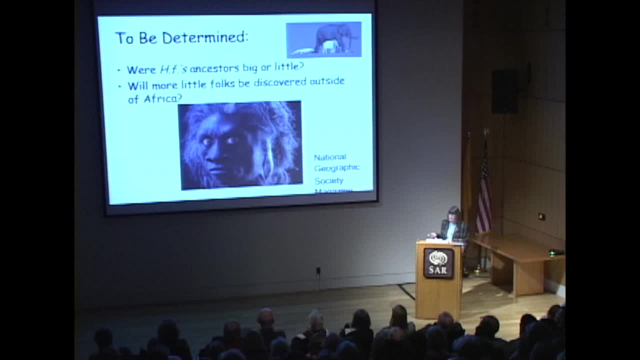 because of things that happen on islands. and where did they come from? Did they come from Java? Were they homo erectus? Or did they some people now think, did they come from Africa, In which case it wasn't just you know. 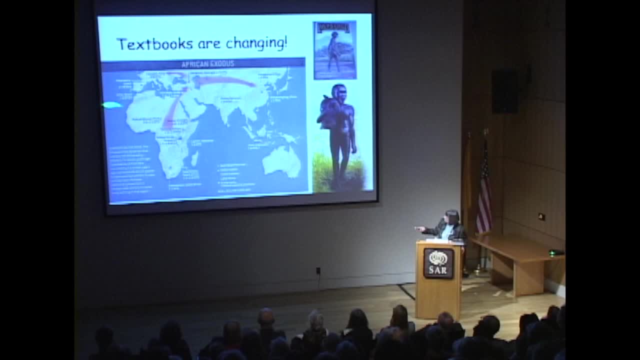 long, tall homo sapiens who left Africa two million years ago. There are hints that maybe australopithecines or their descendants, who weren't yet homo erectus, left Africa around that time too. There are hints, for instance, in the Republic of Georgia. 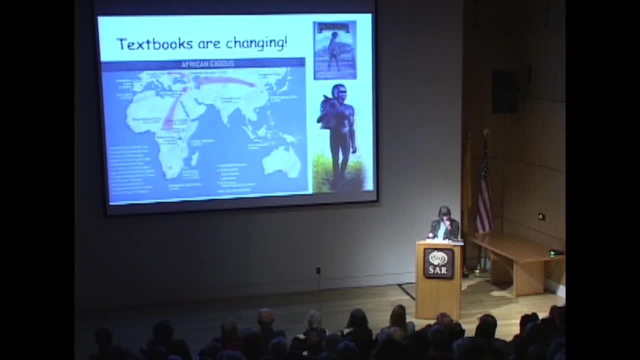 There's some skeletons there that look pretty small and pretty transitional. So the textbooks are now changing and it's been quick. You know it was announced in 2004,, just turned 212, and textbooks are incorporating this, largely most of them. 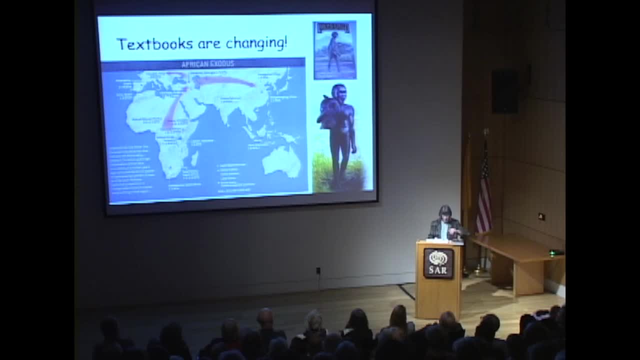 as a legitimate new species. So I think I have a minute or two. I want to bring you up to revolution number three, which is just starting, And it actually speaks a little bit to homo floresiensis, And this has to do. 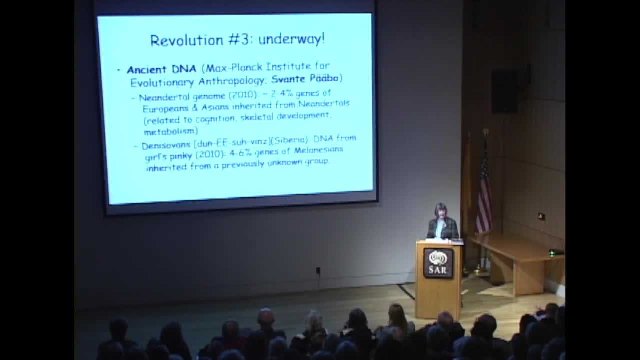 with genetics, And it's the Max Planck Institute for Evolutionary Anthropology in Leipzig where this is going on, And the genius that's been doing the work- his team- is Dante Paabo, And what he's perfected is a technique for extracting DNA. 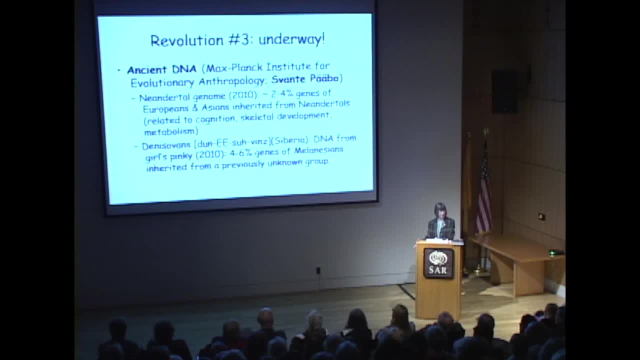 from fossils- with luck, assuming they're not contaminated and they were found in a cold enough place- and then amplifying it and then comparing parts of the genome in chimpanzees and people from around the world and in the fossil and seeing what the evolutionary 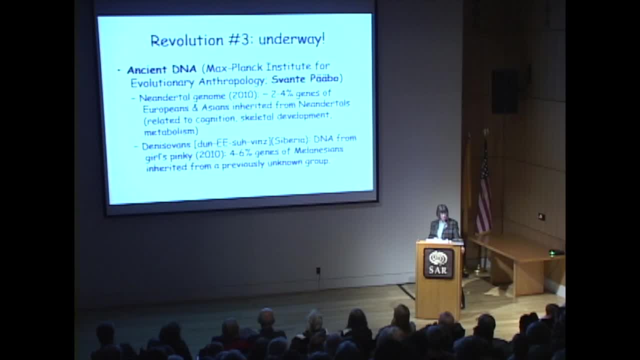 relationships were They had? I think in Leipzig they actually had a bias. I mean, I've thought that for some years where they were, like much of the field, biased against poor old Neanderthals who you know. 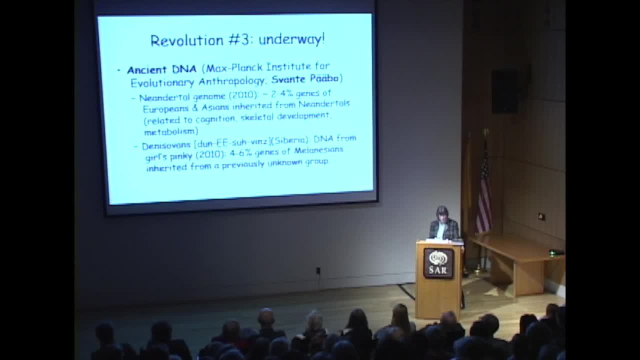 they weren't our ancestors. That's a whole other story, And they initially published that. that's what their genetic studies told them. However, the big one- the genome- came out fairly recently, in 2010., And they went hold it. 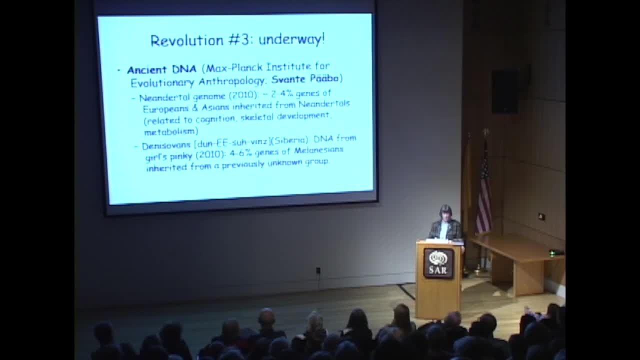 We see now that in living Europeans and living Asians that two to four percent of their genes seem to have been inherited from Neanderthals. So they had to do some backtracking, And boy did they. they were meticulous in their analyses. 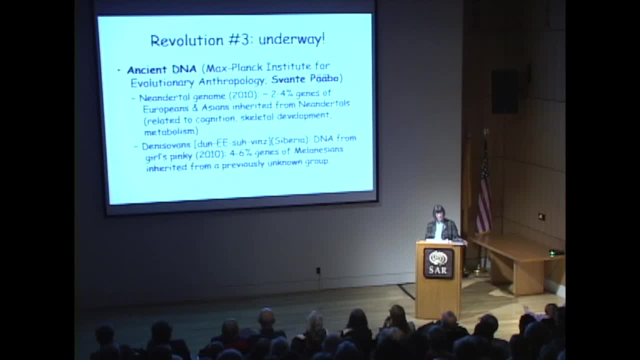 Meticulous. So this some people love it because there have been debates about out of Africa and whether or not Neanderthals have anything to do with our genome And this suggests that they do indeed. Also, they were able to identify in living people. 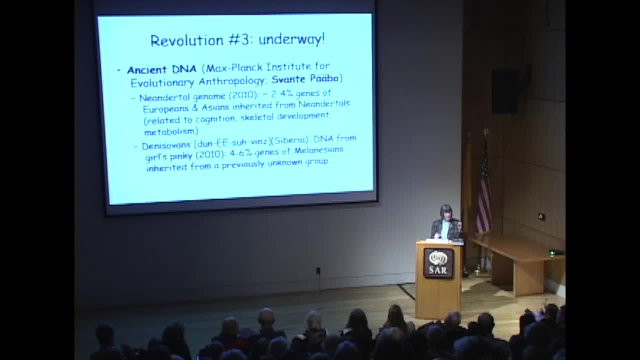 parts of the genome that had evolved, compared to Neanderthals, since they split some hundreds of thousands of years ago. There's a handful of genes And those genes, some of them, they know the function, Some of them relate to skeletal development. 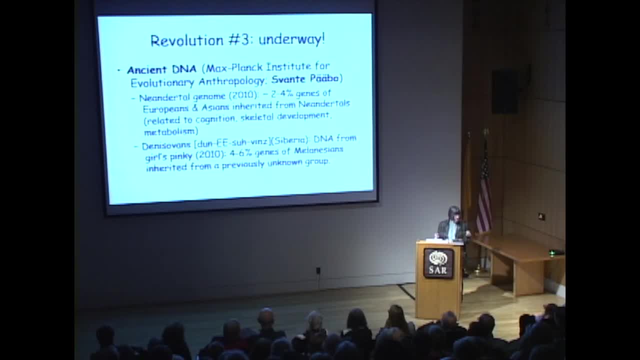 And if people get a mutation, a bad mutation- in that gene, they get weird things happening with their skull and shoulders that look kind of like Neanderthals. There's something to do with metabolism and skin color And then, interestingly, 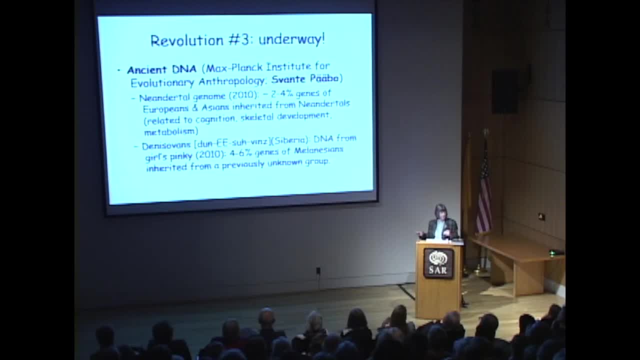 some of the genes if you get mutations in them. in contemporary people suggest that cognition- cognitive things- were under intense selection pretty recently, since the split with Neanderthals, because they're associated with things like schizophrenia and autism. So this is a revolution. 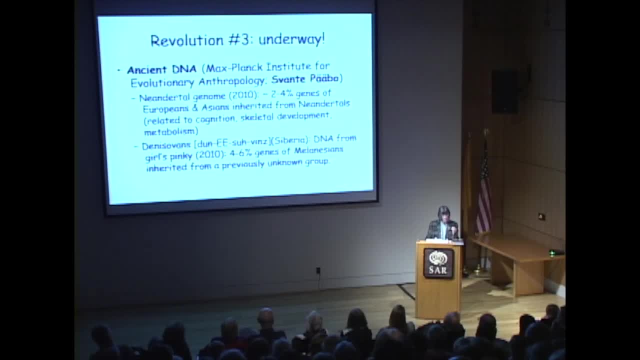 that is just beginning And there's an exciting future here and we'll learn more and more. And the same team, about half a year later, in 2010,, took a little pinky bone from a girl from a cave in Siberia. 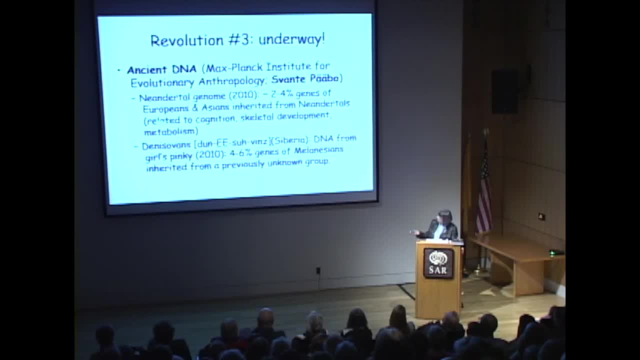 and studied it the same way, And here's the name. It looks like Denisovans, right, But according to the New York Times, it's Denisovans is how we pronounce that- And what they found was that in the Denisovans. 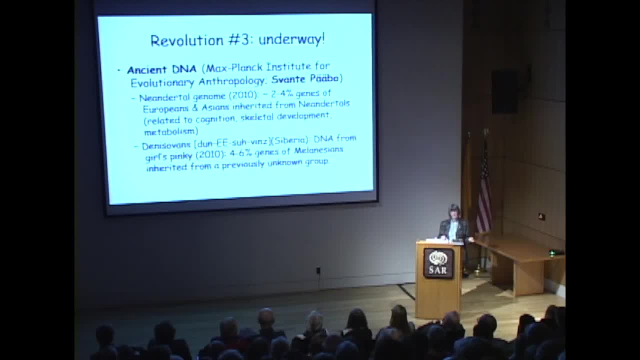 that four to six percent of the genes from people that live in Melanesia are from Denisovans and they have the Neanderthal genes too, But they don't see the two as that related to each other- The Denisovans and Neanderthals. 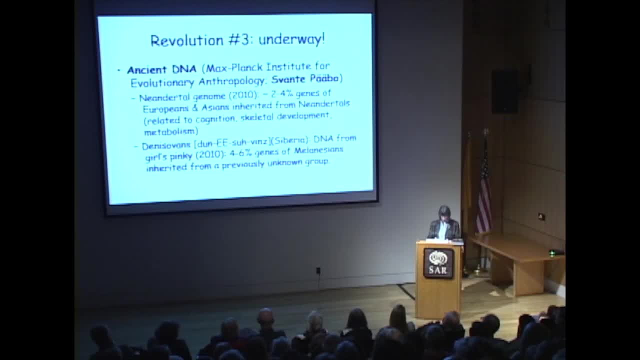 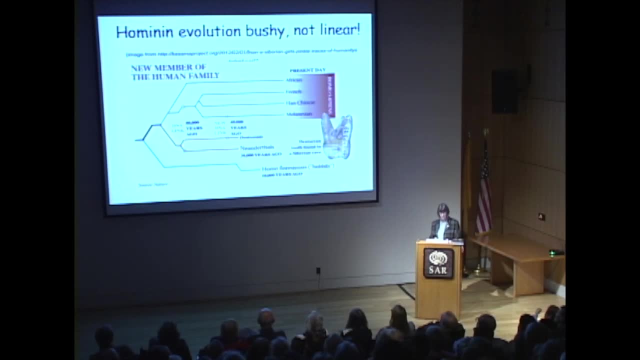 are somewhat related. So what this suggests is, if you look at this, is that what the genetic, new genetic studies are showing, and what Hobbit helped to show is that the idea of the linear sequence of hominids, one evolving into another. 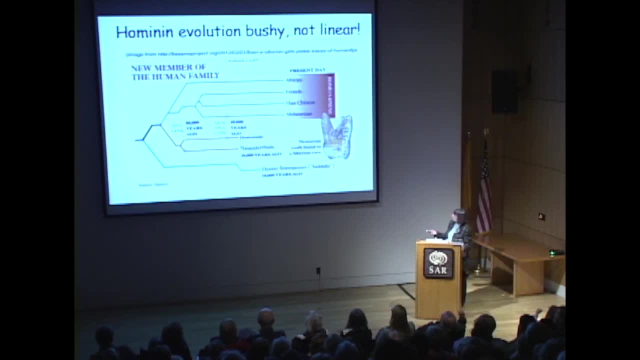 is oversimplified. In fact, hominid evolution, if we go back to about 40,000 years, was bushy. It wasn't linear. When Hobbit was discovered, it was like hey, there shouldn't be anyone other than Homo sapiens. 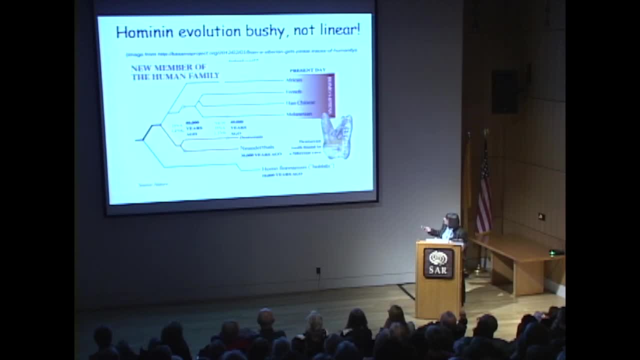 alive on the planet then? But look at that point. you have people all over the old world, You have Denisovans, you have Neanderthals and you have Homo floresiensis, And this truly is a revolution. that's just getting going. 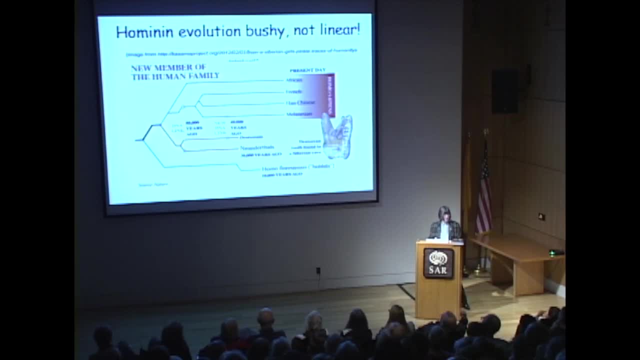 in paleoanthropology, and it's the genetics, that future genetic studies, that are going to give us insights that we probably can't even imagine at this point, And I want to show you a little cartoon that sums this up. This was: 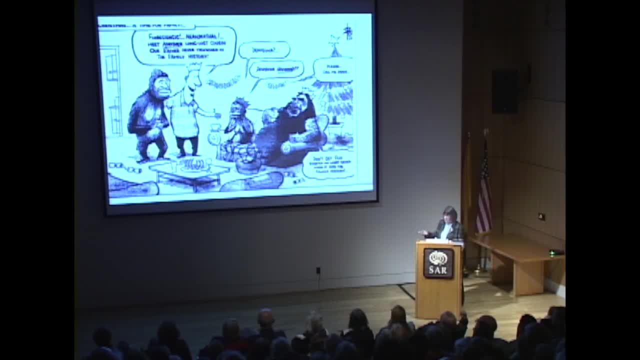 this is Christmas, a time for family, It says up there and we've got over here: floresiensis Neander, floresiensis Neanderthal, meet another long-lost cousin our father never mentioned. 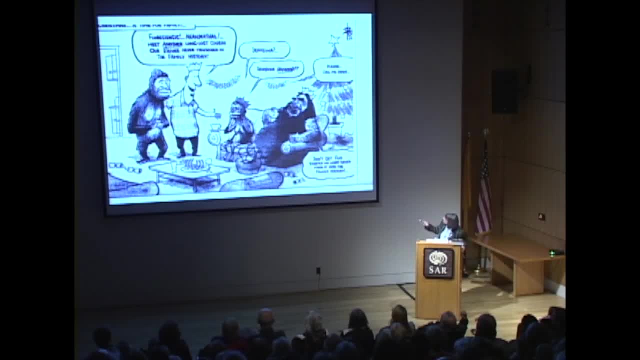 in the family history Dunysuva, Dunysuva, hominid, Please call me Duny. And then the Neanderthal says: don't get Flo started on what never made it into the family history. So that's where the field is. 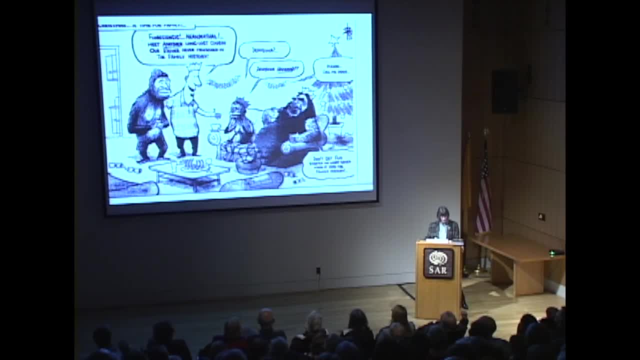 But also I have one other slide Which is not only. I mean, I'm so happy that there's such a good turnout tonight and that people are interested in paleoanthropology and these revolutions, But I'm delighted that these genetic studies. 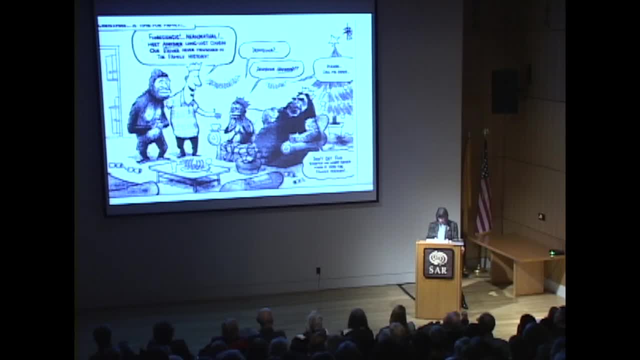 are revolutionizing not only the field, but also advertising. One of the things that came out of them was that Neanderthals were probably red-haired- Go figure- And light-skinned with freckles, And so it's affected. 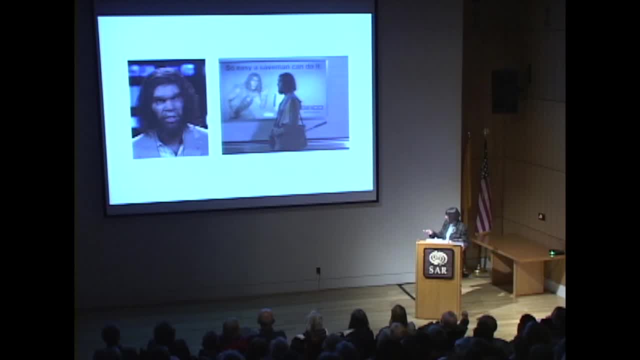 it's revolutionizing advertising. I don't know if you noticed- only his hairdresser knows. but the Geico caveman suddenly has red hair And I'd like to think it's because all those advertising folks are sitting around reading Nature and Science. 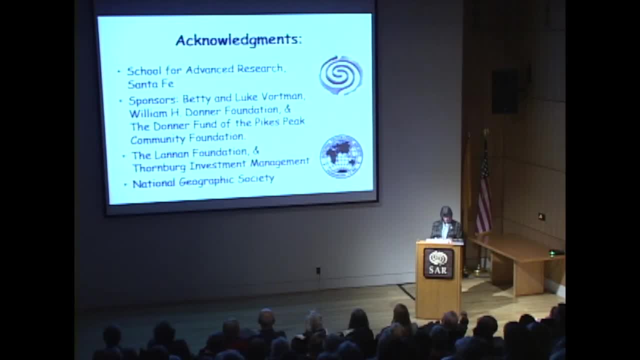 Thank you so much for your attention. I want to again. I want to add to James' acknowledgments For this evening for the support, But first of all I want to acknowledge so much SAR for their support. I am thrilled. 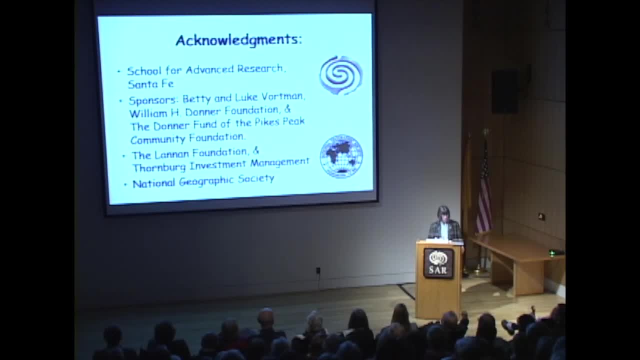 to be associated with them And I hope- James, you're right, I hope it goes on for a long, long time- And our sponsors- again- he mentioned them, but you can never mention them too often- Betty and Luke Fortman. 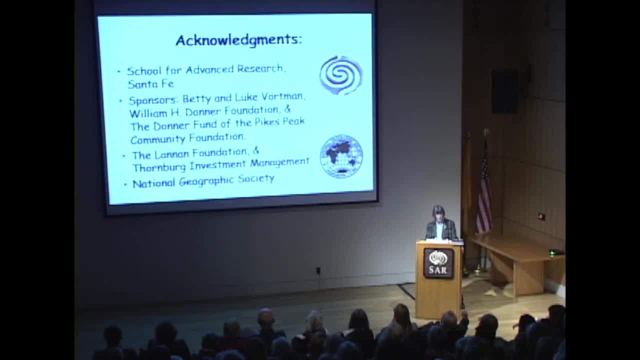 the William H Donner Foundation and the Donner Fund of the Pikes Peak Community Foundation. Also other supporters of SAR, the Lannan Foundation and the Thornburg Investment Management. And I also want to acknowledge National Geographic's support of our research. 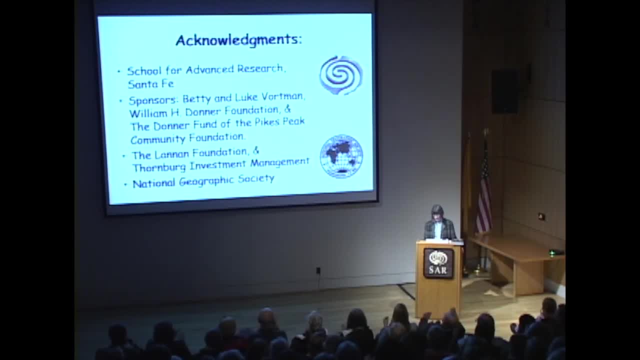 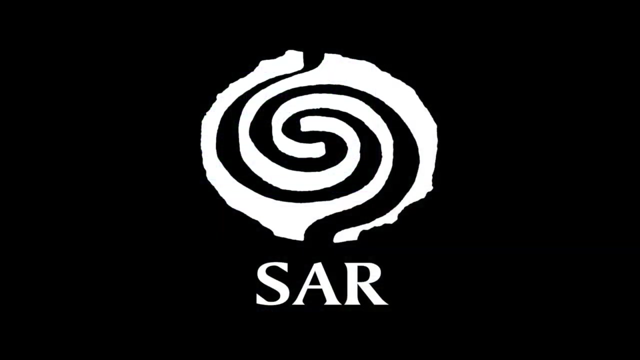 on Homo floresiensis. Thank you, Thank you.